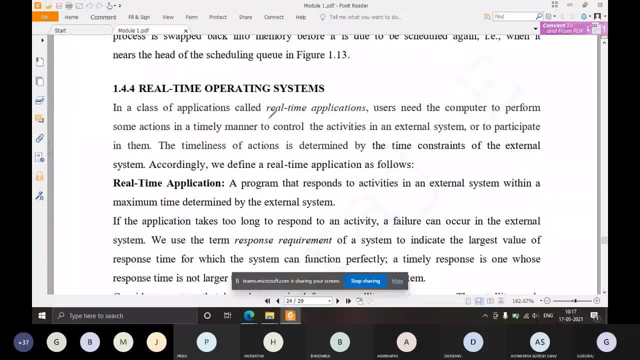 operating system. Missing that deadline may result in catastrophic results. It may result in irrecoverable damages. For example, if you take the braking system itself, if it does not respond to your command of applying the brakes, then there may be a loss of life or loss of many lives. That 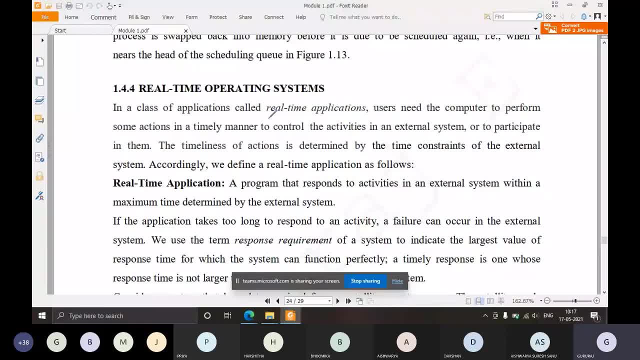 is why the deadline should be satisfied. Otherwise it will result in a catastrophic result or irrecoverable damage. Such type of systems are known as real-time systems. These real-time operating systems are applied in real-time applications. Users need the computer to perform some actions. 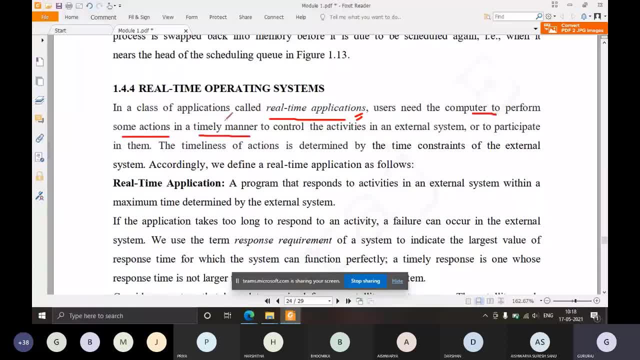 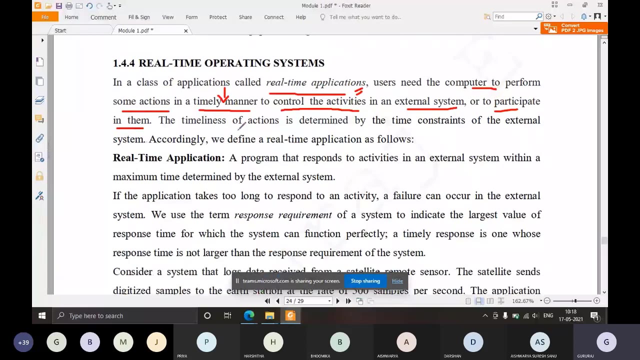 in a timely manner. You can see the word here: timely manner Every time that system has to respond within a deadline, or it has to perform an operation in a timely manner to control the activities in an external system or to participate in them. The timeliness of 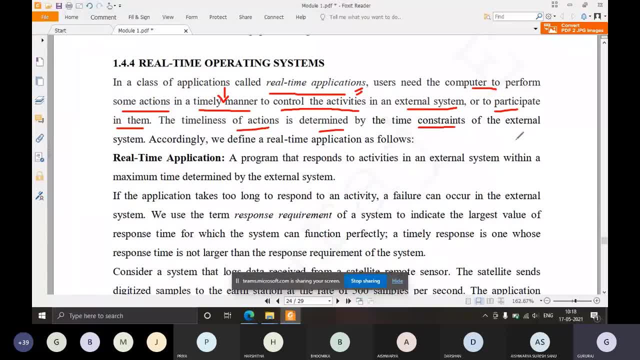 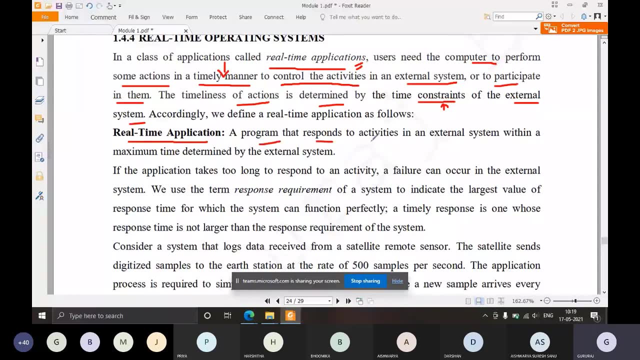 actions is determined by time constraints. There is a time constraint, nothing but deadline, for the external system. So real-time application. So what do you mean by real-time application? A simple definition: A program that responds to activities in an external system, For example, 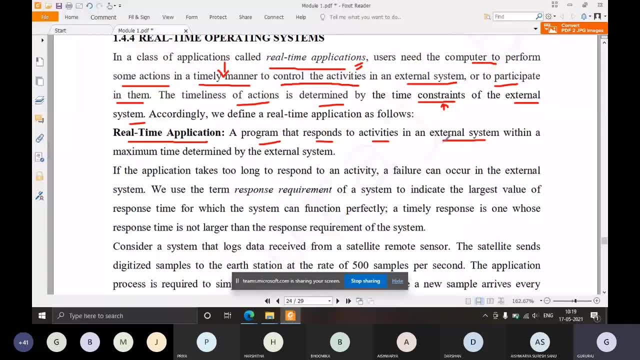 a program that responds to activities in an external system within a maximum time determined by the external system. This maximum time is nothing but deadline, So that application has to respond within the deadline given, within the maximum time specified. Suppose there is a system wherein the output, once you give the input, the output should be available. 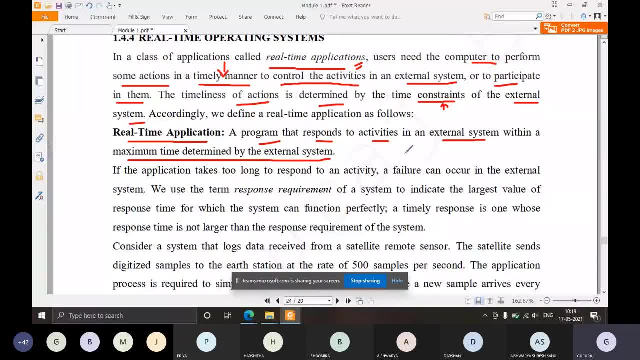 within, let us say, 10 milliseconds, So that program or the operating system has to respond in such a way that every time the input is given, the output is available within 10 nanoseconds or 10 microseconds. So missing this deadline may result in an unrecoverable damage or unrecoverable. 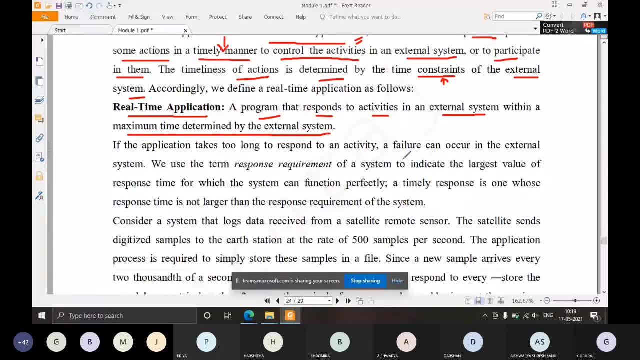 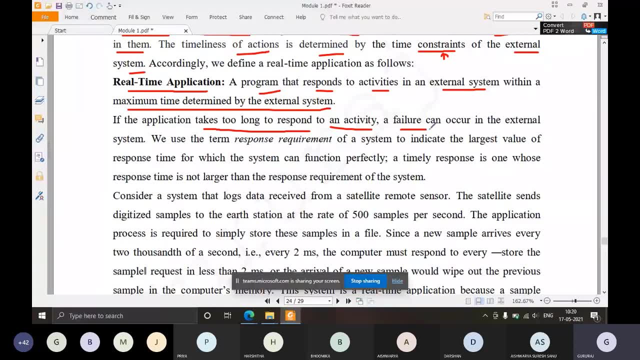 loss If this application takes too long to respond to an activity. a failure can occur in an external system. That is the word. If the deadline is missed, so that will result in a failure. So this failure- we use the term response requirement of a system to indicate 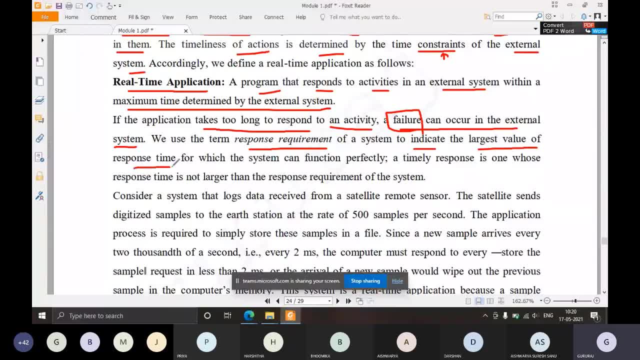 the largest value of the response time for which the system can function perfectly. So there is always a largest value of the response time, nothing but the deadline within which the system can perform perfectly. If the time response is missed, so then it may result. 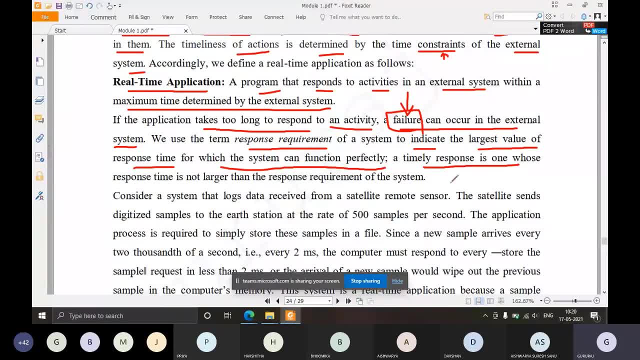 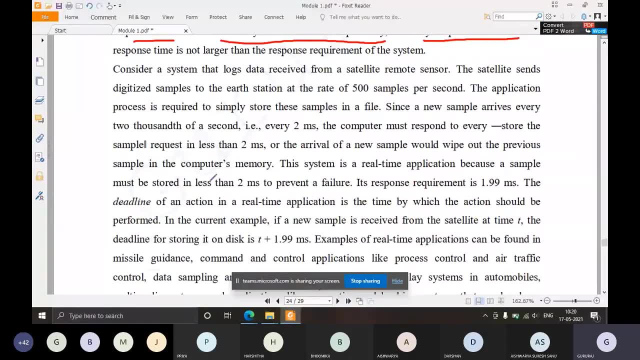 in a failure or it will result in a failure. It is not may, it is definitely it will result in a failure. So example one example is discussed of a real-time system. Consider a system that logs data received from a satellite remote sensor. 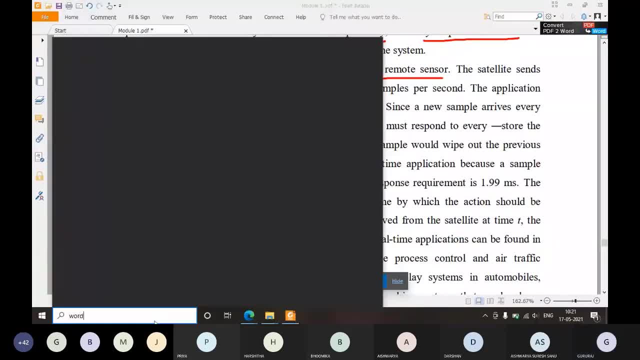 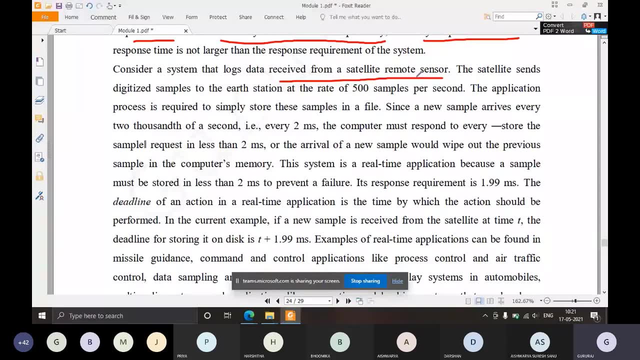 We have to consider a system that logs data received from satellite remote sensor. logs means, whatever the data that is received from the satellite, that data will be saved onto a memory. That is what we mean by log the data And this. there is a system which. 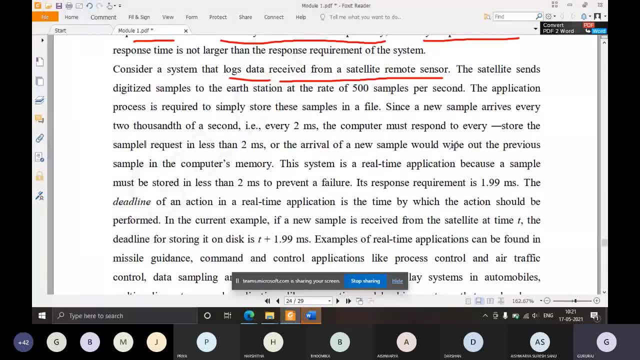 is on the earth and the satellite is in the space. We have to consider a system that logs data from a satellite remote sensor. So logs means So the satellite is sending some data from the space to the system on the earth. So it is a wireless communication that is happening or it is a satellite communication. 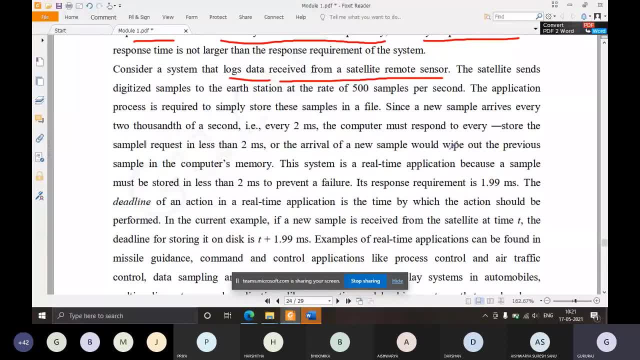 that is happening. So the system on the earth, so what it has to do: Whatever the data sent by the satellite, it has to store that data somewhere in the memory. So the satellite sends digitized samples to the earth station at the rate of 500 samples. 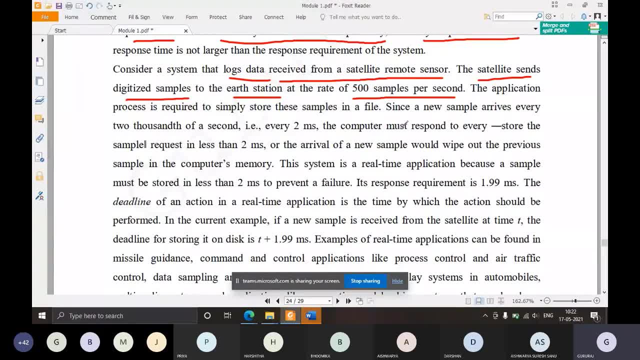 per second. So see here, the satellite is sending the data at a rate of 500 samples, and these are digitized samples, nothing but zeros and ones. so at a rate of 500 samples per second, every second, the system that is available on the earth. it is receiving 500 samples. 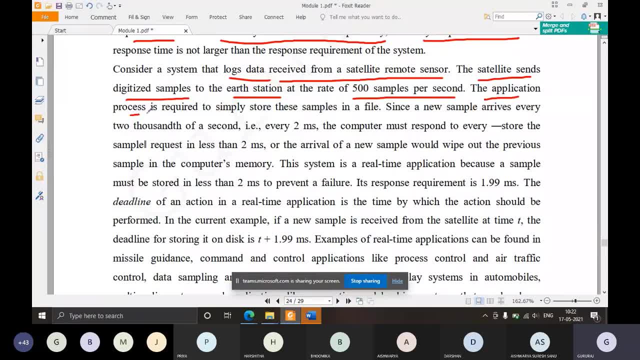 So the application process is required to simply store these samples in a file. This is what is the application. so you have written a program that is there on a system on earth which is receiving the data from the satellite at a rate of 500 samples per. 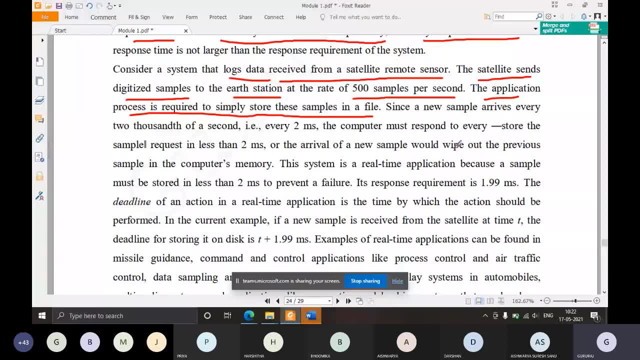 second. So whatever the program that you have written, it has to simply save all those 500 samples onto a file. Okay, Onto a file, Since a new sample arrives every two thousandth of a second, that is, every two milliseconds. 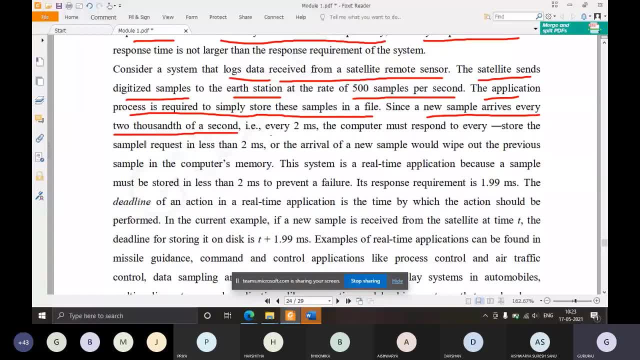 so what he says? 500 samples per second means one sample will arrive at every two milliseconds. that is what that is the meaning. 500 samples per second means you are receiving a sample, a digitized sample, from the satellite Every two milliseconds. 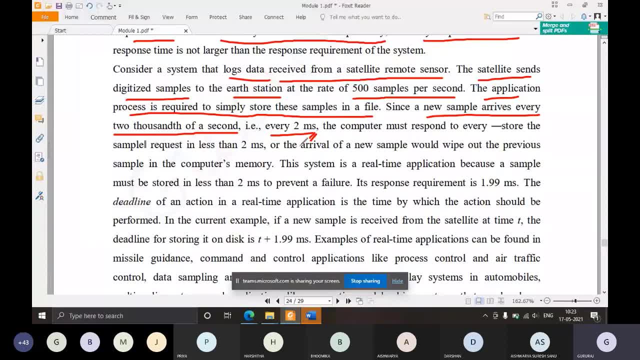 That means what? what is the meaning of that? So two milliseconds is the deadline and two milliseconds is the deadline. So what is the? what do you mean by deadline? Whenever you receive one signal, okay, one digitized sample, so what will happen is: 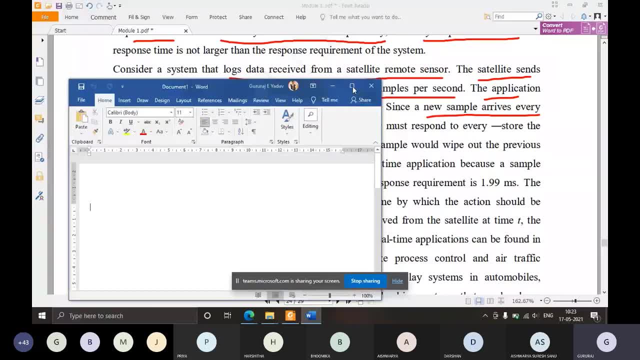 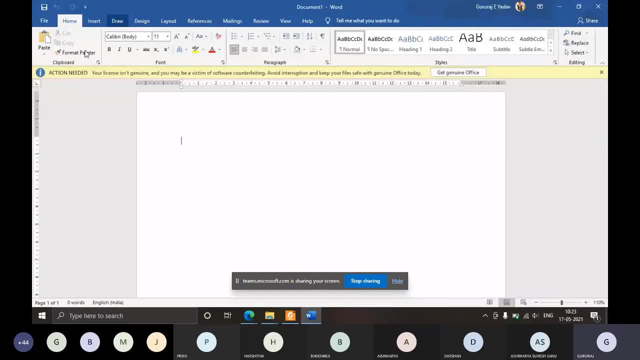 as soon as you receive one digitized sample. so what will happen is so the system that is available will arrive and will show a list of the samples, And that is what you call passive sampling. Okay, That is your dels –uh. 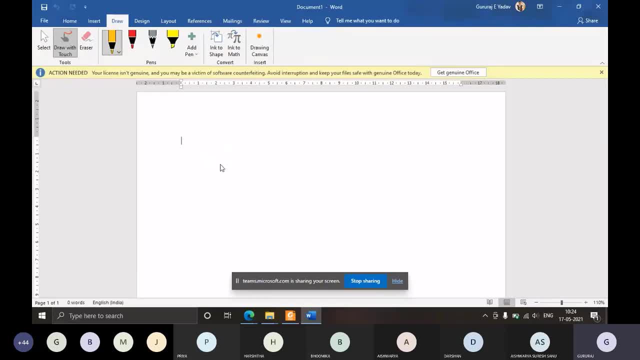 Climate? Yes, Is it actually as navigational? yes, 데u petri, but has the artifact the best piece? Okay, that is the system that is on the earth and there is a program written on that. okay, so this is the system on the earth and this is the satellite. okay, so this. 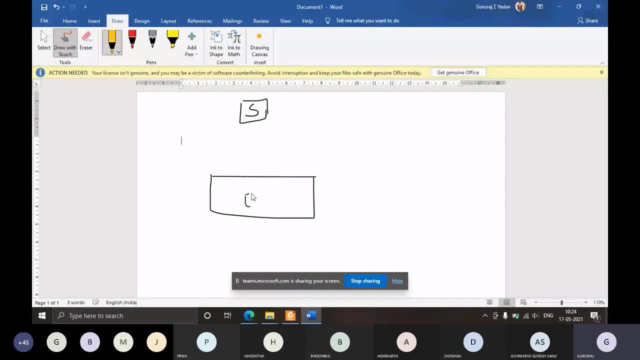 is in space, this is the system on earth. so in this system you have written a program. okay, so this satellite is sending wireless. the wireless is sending some samples at a rate of 500 samples per second. so this implies the system on the earth is receiving actually one sample every two milliseconds. 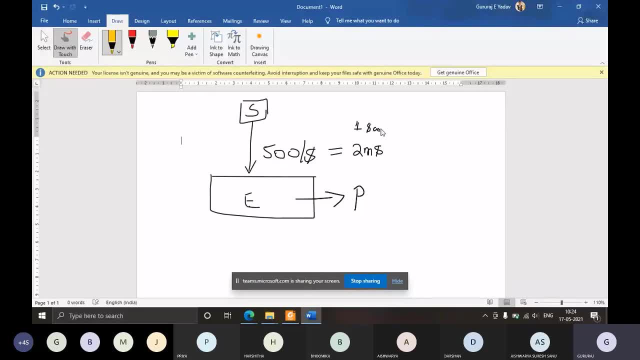 okay, one sample every two milliseconds. so that means two milliseconds is the deadline for the program that you have written to store. to store one sample. okay, so this program will store the data onto a file. okay, so it has to store the data onto the file, and what is the deadline given? 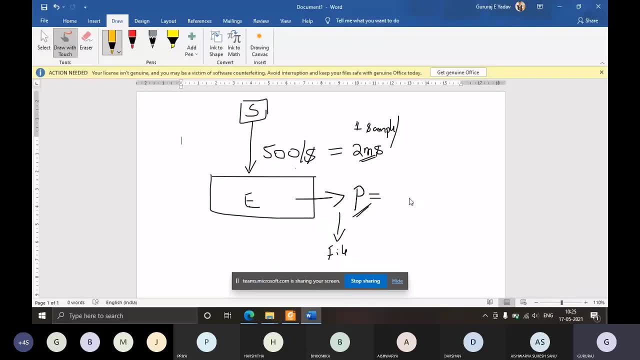 to this program to store one digitized sample. if the deadline given is two milliseconds, within two milliseconds it has to store that digitized data onto the file and it should be ready for receiving the next sample. okay, next sample. so every two milliseconds it will receive the sample, okay. 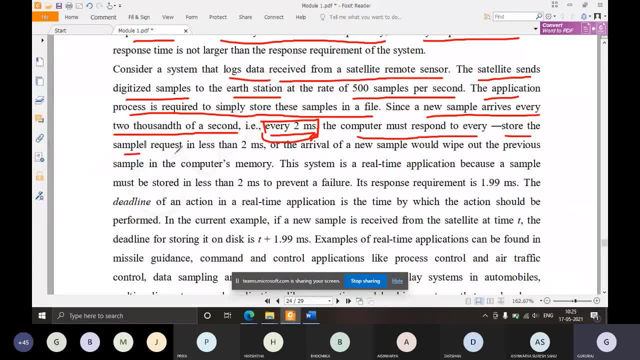 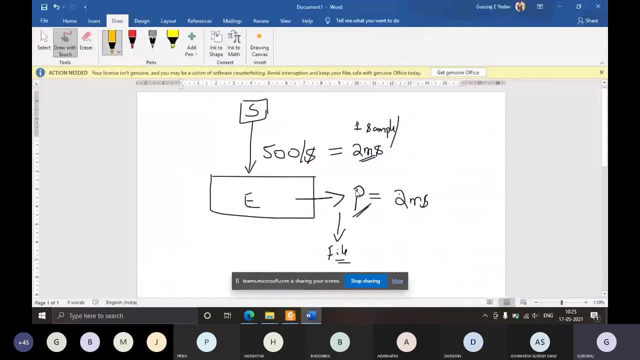 the computer must respond to every store the sample request in less than two milliseconds. okay, so that is what I. two milliseconds is the deadline within two milliseconds. this program has to store the digitized sample received from the satellite onto a file and it should be ready to receive the next sample. and 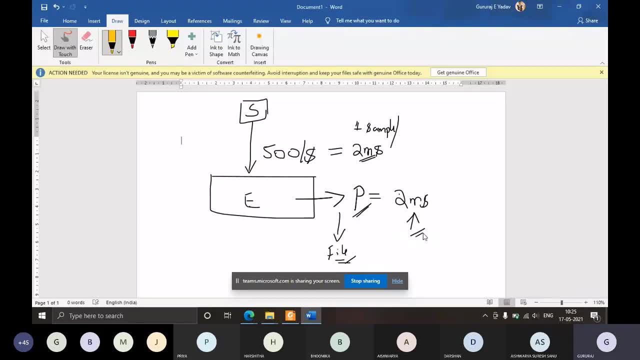 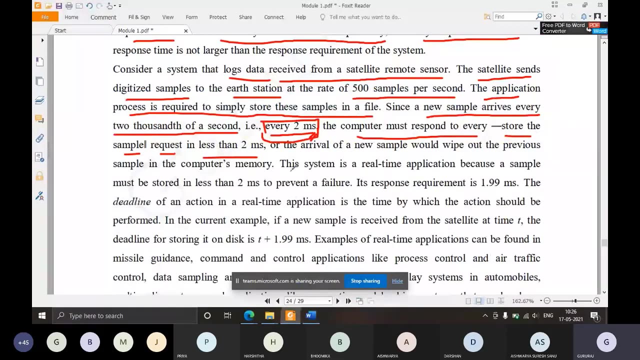 this should. everything should happen within two milliseconds. two milliseconds is the maximum time, okay, this is what you call as deadline. this is the deadline, okay, so we shall see what will happen. if this is not satisfied, restore the request, okay, or the arrival of the new sample would wipe out the previous sample in the computer. so what will? 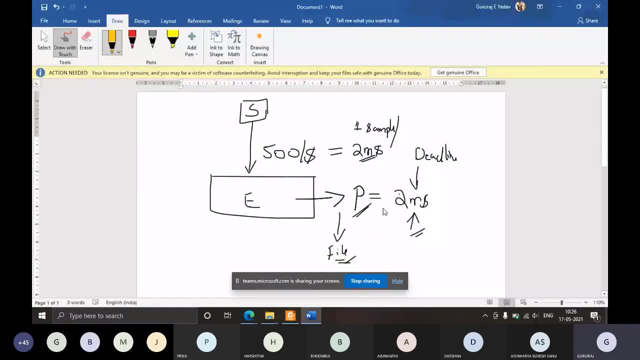 happen if this deadline is missed, if this program will not store the sample received by the satellite within two milliseconds, then what will happen is, within the within the completion of storing this, the next sample will arrive. next sample from the satellite will arrive, and what it will do is it will overwrite the previous. 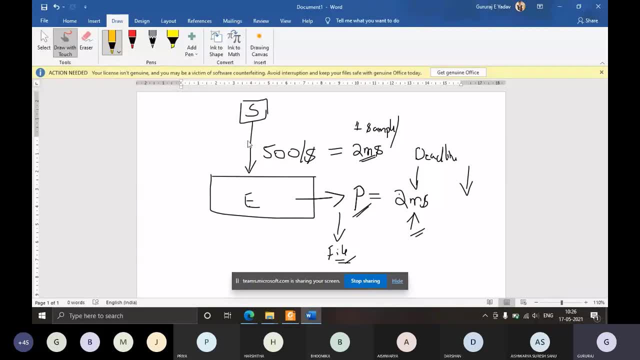 sample because, see, usually what will happen is the sample can be 8 bits or 16 bits. let's say it is 8 bits, okay, so whatever the sample that is received by the satellite, let's say each sample is of 8 bits. so to receive this, there will be a 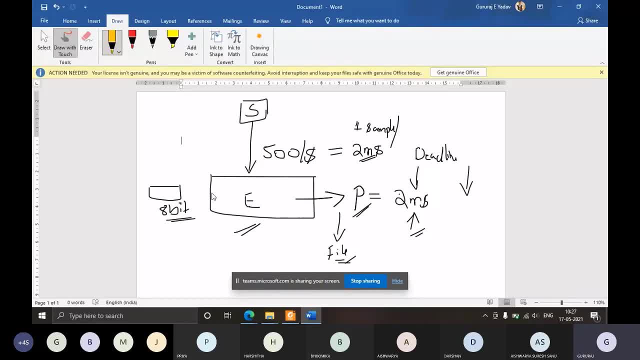 buffer in this system which is on the earth. so there is a buffer. this is known as a buffer, it is a temporary storage, okay. so this buffer, it will receive the sample from the satellite, okay, and it will be temporarily stored here until it is written or stored to the file. so who will do this job? so the program that you 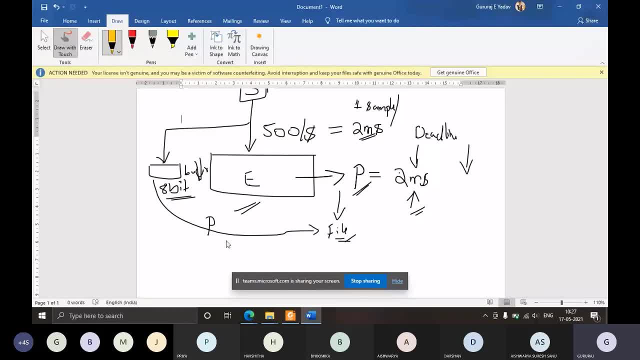 have written will do this job. what it will do is it will fetch the 8 bits stored in this temporary buffer and it will store that file and- sorry, it will store that data to the file. and this should all happen within two milliseconds. so if this does not happen within two milliseconds, what will happen is the next. 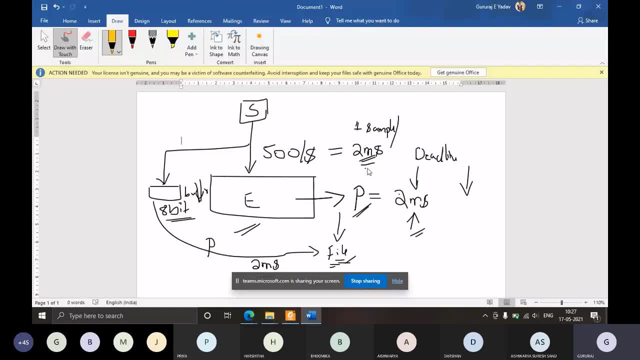 sample will arrive from the satellite, because every two milliseconds the next sample will arrive. and the next sample, when it arrives, it will be again stored on the same buffer, because there is only one buffer here, 8 bit buffer. so the next sample will also be stored in the same buffer. so, before the next sample arrives, if this store operation is not completed, 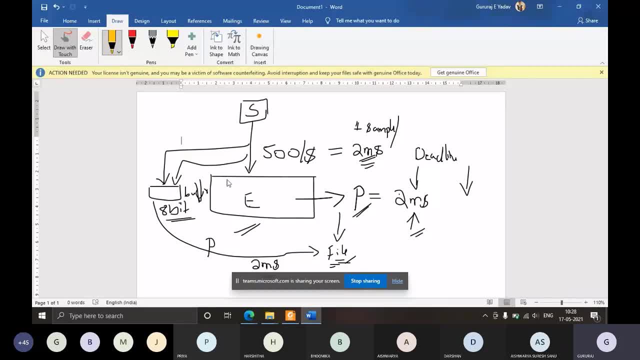 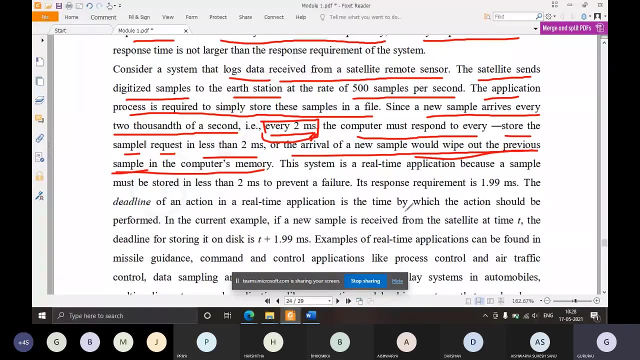 then what will happen is the previous data that was there. it will be overwritten by the new sample. so the new sample will overwrite the previous sample. so this will result in loss of data. okay, so that is would wipe out the previous sample. loss of data. so this system is a real-time application, because a sample must be stored in less than 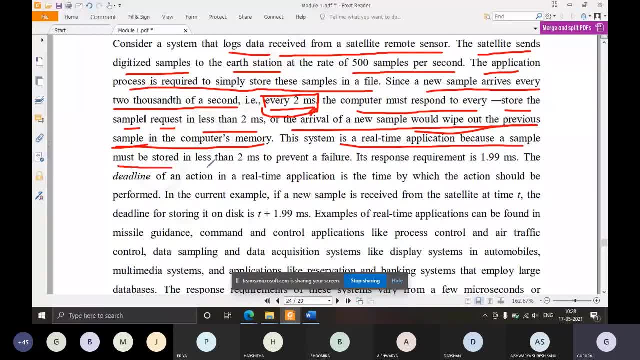 2 milliseconds to prevent the failure. so failure is loss of data. okay, its response requirement is, let's say, 1.99 million. everything that is the store of each digital data, should happen within two milliseconds. so that is why the deadline is taken as one point. 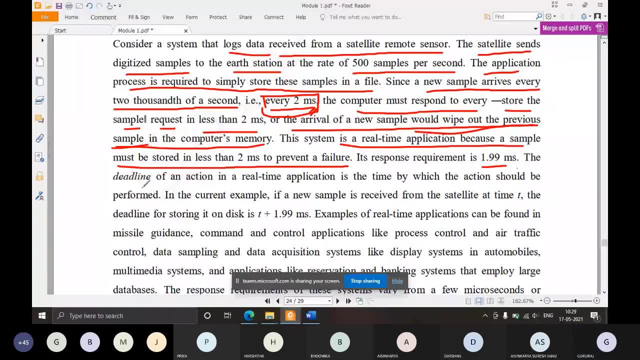 So next, the deadline of an action in a real-time application. So what is the deadline? It is the time by which the action should be performed. That is what we mean by deadline. It is the time by which, whatever the action of that application should be performed. 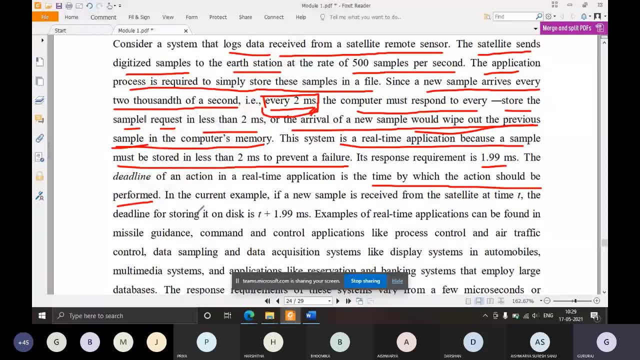 In current example, if new sample is received from the satellite every t milliseconds, the deadline for storage onto the disk is t plus 1.99.. So every 2 milliseconds you are receiving the data means the deadline will be 2 plus 1.99 milliseconds. 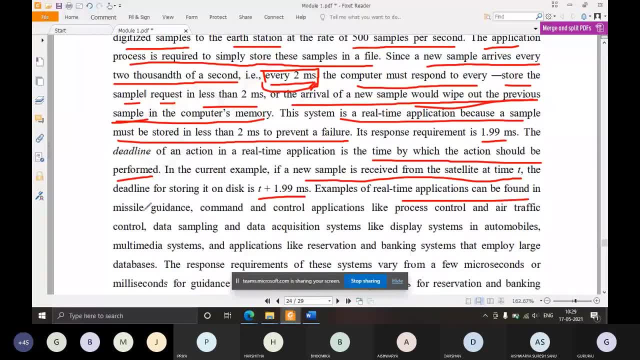 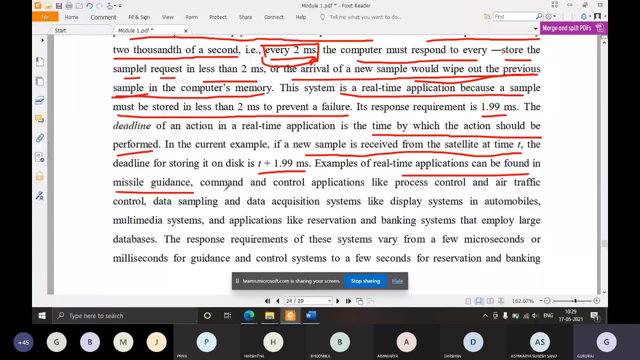 Examples for other real-time applications can be found are: so one is in Mizzle Guidance, So there is a microcontroller or a processor that is fitted onto a missile. So every missile will contain that because it has to accurately reach the target. It has to accurately hit the target and destroy the target. 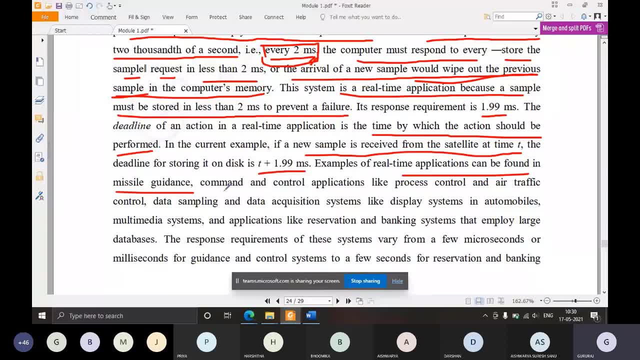 So for that accurate destruction of the target, so it should be real-time. So, whatever the systems that are used on the missile, It should be real-time. the tracking of the missile, the speed of the missile, everything should be real-time. 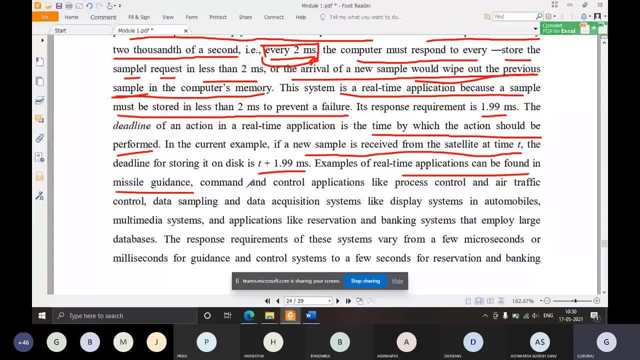 Otherwise, what will happen is if that deadline is missed, it will go and hit somewhere else. It will go and destroy some other target which was not supposed to happen. So again it will result in loss of lives, because if you don't hit the target properly, 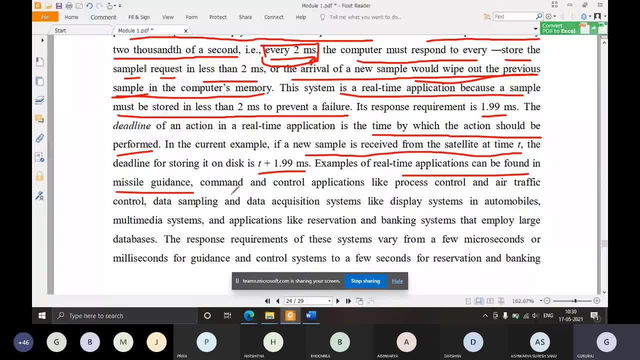 then the satellite will go and hit some other- you can say place- So it can be full of people- and it will be resulting in loss of lives. So that is one example. Next is command and control applications like process control and air traffic control. 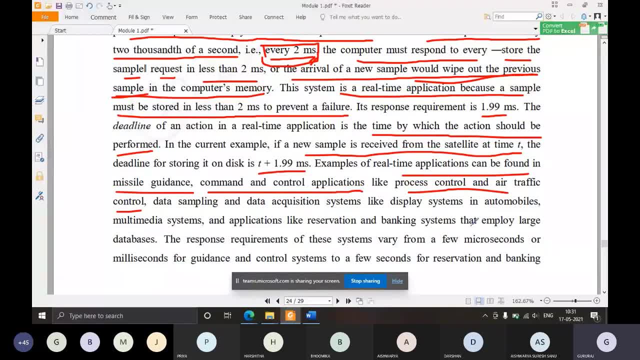 So this is again very important- Air traffic control- you might be familiar with air traffic control, which will control the operation of the flights that are, let's say, commuting throughout the air traffic control. Okay, so there is a air traffic control for every country. 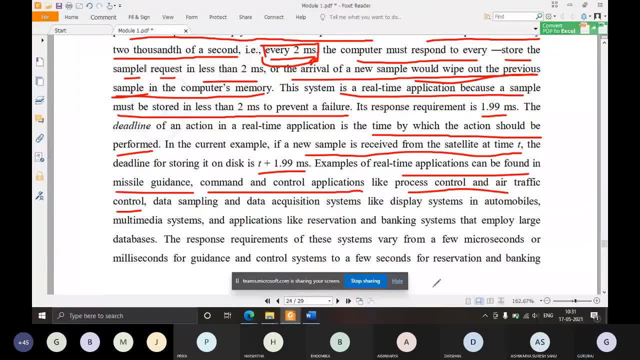 So for India, they are having one air traffic control. for America, they are having one air traffic control which will monitor regularly where is the plane okay, and at what distance and what altitude is the plane at the present. because this tracking is very important, because 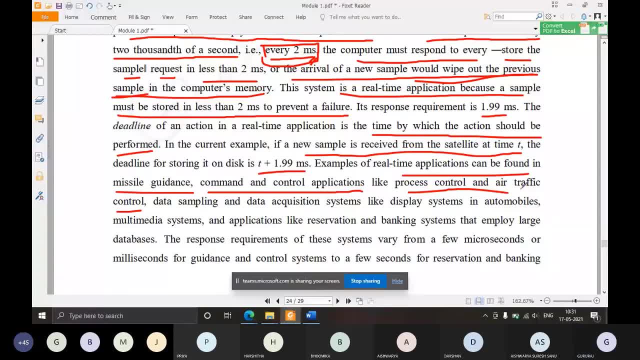 no two planes should collide with each other, So they should be made aware about the situation of other planes also, so that they will not collide with each other. So hence it is also a real time application, because if you lose track of any one plane, 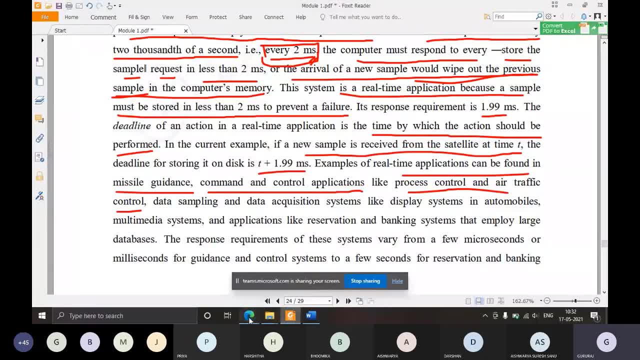 then that will result in loss of many lives. So that is what is air traffic controller will do. Next is data sampling and data acquisition systems: Display systems in automobiles, multimedia systems, applications like reservation and banking systems that employ large databases. Okay, so these are all real time applications. 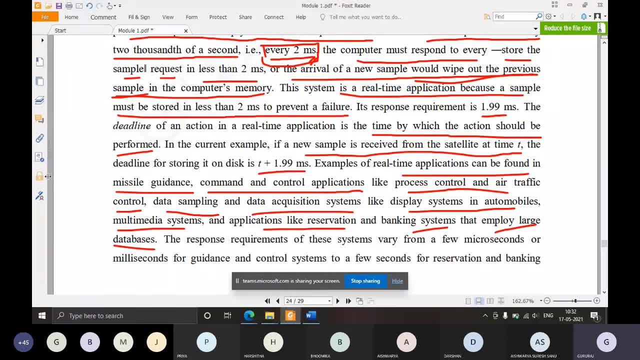 The best example, as I told you, is missile guidance and air traffic control, wherein you have to keep track of the satellite or the plane at every given time moment. Okay, so every millisecond you have to apply, update the data. 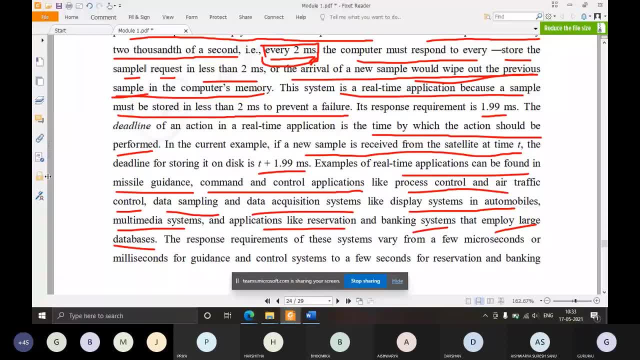 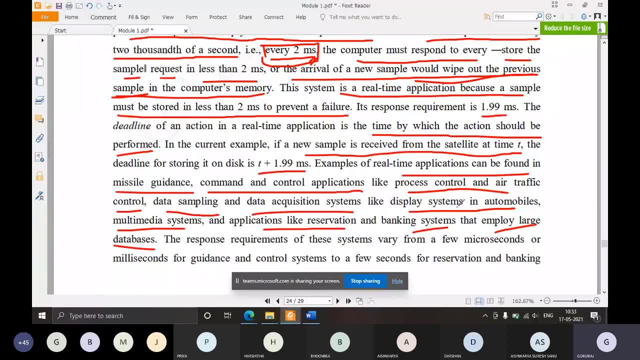 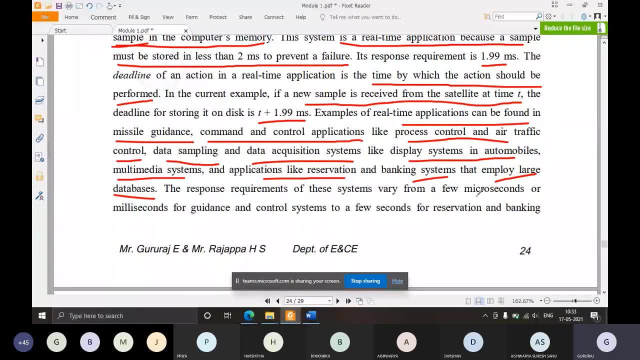 So these are known as real time systems. The response requirement of these systems vary from few milliseconds or microseconds to milliseconds. Okay, so the response time depends on the application. So it depends on the application. Okay, So the response time depends on the application. 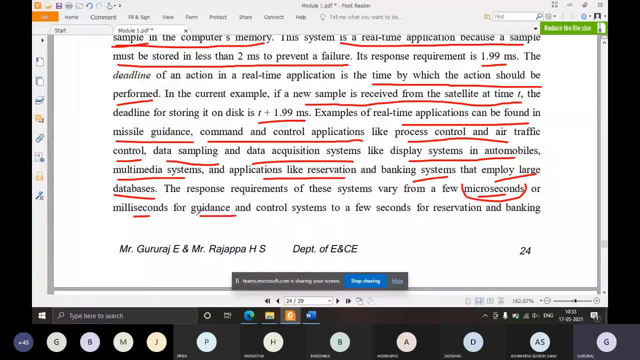 So it depends on the application. Okay, and you can see that the response time is very short. It can be in terms of microseconds. You can see microseconds. It is usually in terms of missile, missile guidance. It is in terms of microseconds because the missile will be traveling at a very high speed. 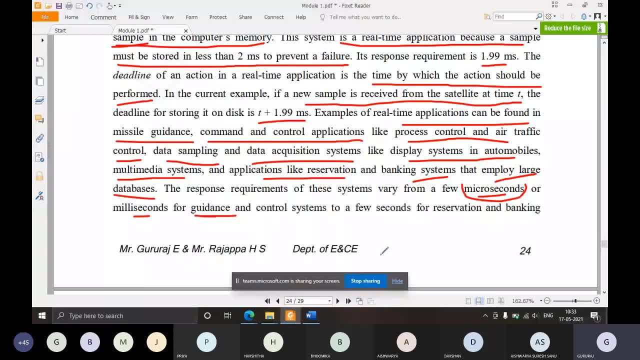 And so it has to keep track of where it is, the- you can say, the location information. it has to keep track because even a slight delay or a slight miss will will result in the target being not destroyed, yes, or a miss hit, so it will go and hit some something else. 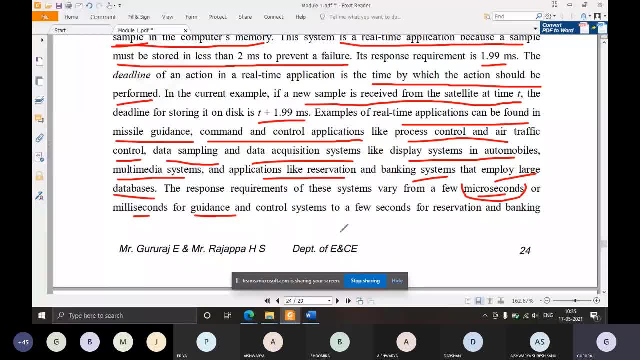 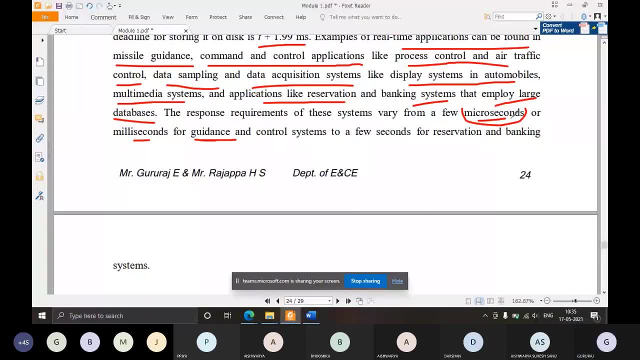 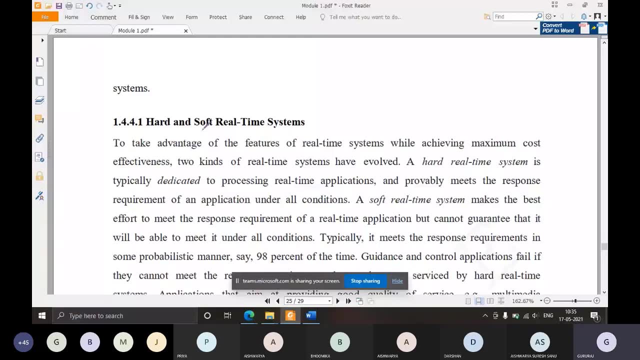 which should not happen in defense. okay, yeah, so that is what is: response time: microseconds or milliseconds? so next there is a classification done in real-time systems. one is hard real-time and one more is soft rate. so you will see what is this to take advantage of the features. 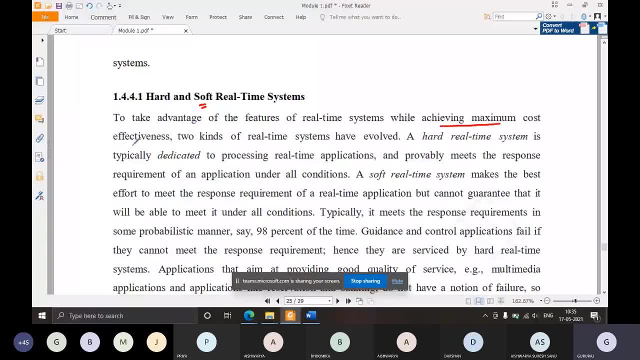 of real-time systems while achieving maximum cost effectiveness. two kinds of real-time systems have evolved classifications: okay, so a hard real-time system. so the name itself is indicating. hard real-time means it should not miss the deadline. okay, so every time that deadline should be satisfied, that is what is known as hard rate. it is typically dedicated. 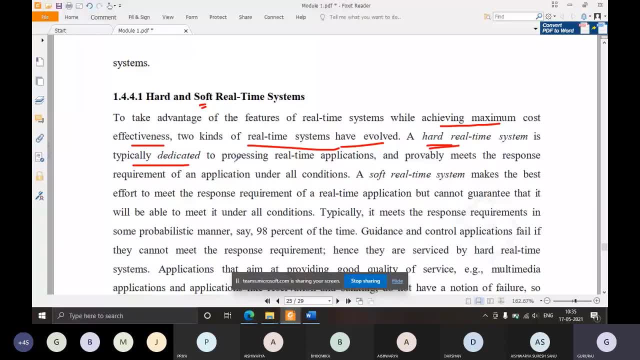 to processing real-time applications and it probably makes it possible for the system to meet the response requirement or the deadline of the application under all conditions. so every time, but at any cost, at any condition, the real-time system should meet the deadline. so such type of systems are known as hard real-time system. okay, so what about soft real-time? 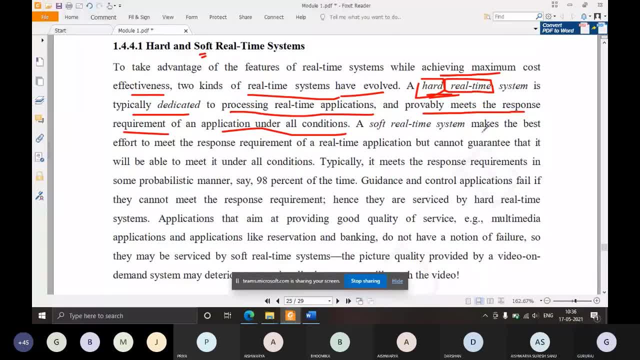 soft real system. real-time system makes the best effort in the application. so this is a soft real-time system that does not guarantee that it will be able to meet the deadline at all conditions. okay, so that is soft rate, so soft real time. it puts its best efforts. 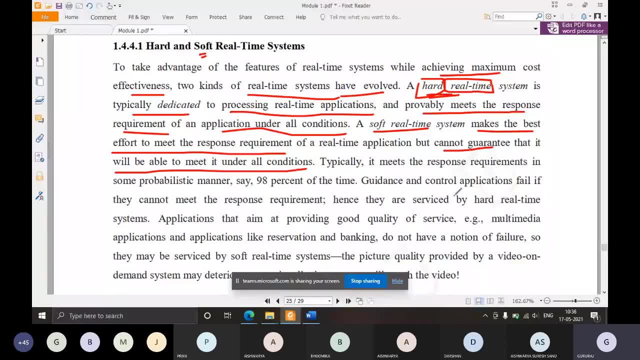 to meet the deadline, but it does not guarantee, or it will not guarantee that it will not guarantee that it will be able to meet the deadline at all conditions. Okay, so I'll give you an example for this: hard real time and soft real time. The hard real time is so I have. 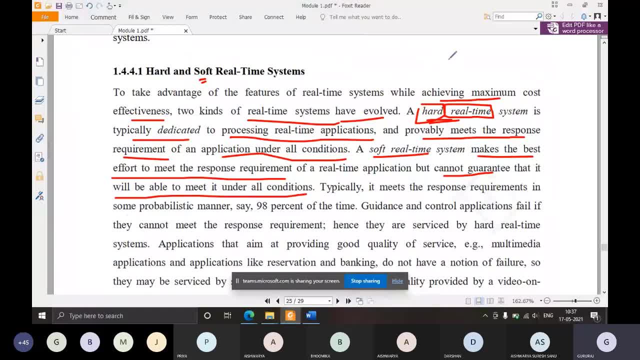 given an assignment for you people and you have to submit the assignment by, let's say, tomorrow, before 1130.. Before 1130.. So an assignment is given and the students have to submit the assignment by tomorrow, 1130.. Yeah, Within within this. 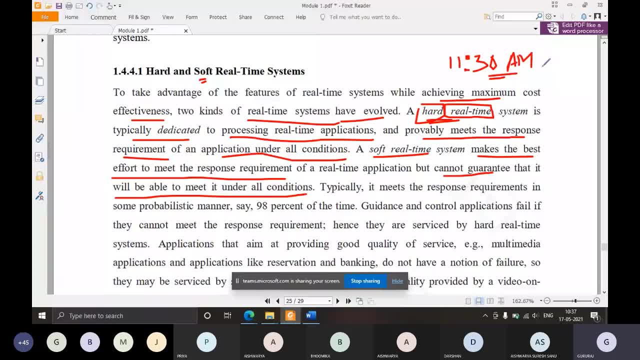 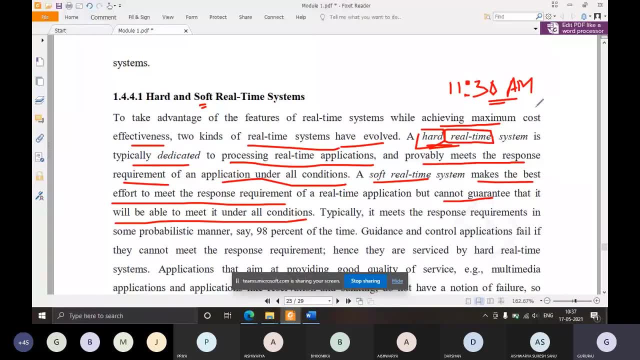 deadline, that is, 1130, am to whoever submitted the assignment that those will be considered for evaluation. And after 1130, after 1130, whoever submits they'll not be considered as as the for, how you can say, for the evaluation. So in such, in such, 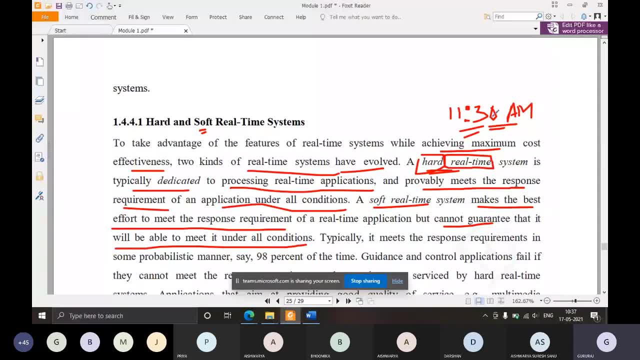 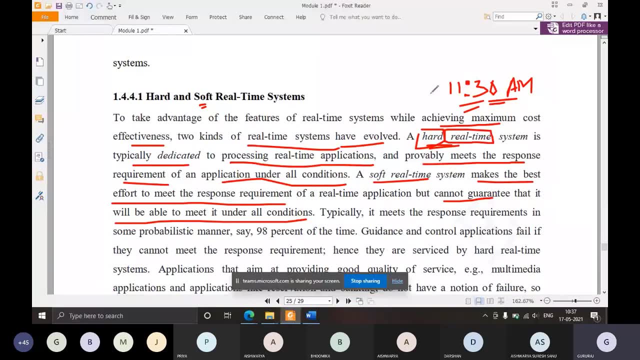 deadlines. see the the. you can say: the policy is a late answer is a wrong answer. This is a very simple policy that is employed in hard real time systems. So what is your policy? A late answer is a wrong answer? Okay, so even though you give the correct answer also, but you 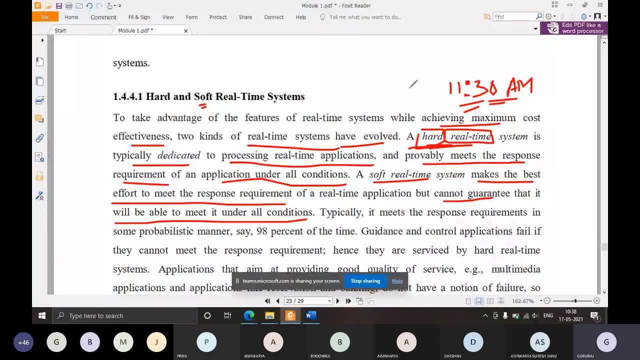 if you give that answer after the deadline, then it is considered to be a wrong answer, And in hard real time systems, if you miss the deadline, then the damage is irrecoverable. Okay, so it will result in a irrecoverable damage. Okay, So that is what is hard real time. 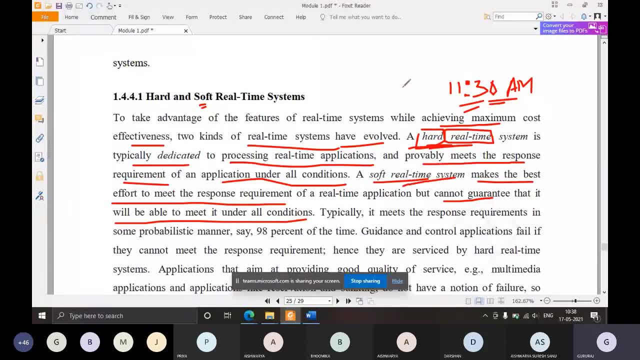 But in soft real time. so the policy is: so a late answer is acceptable answer. it is still acceptable. Okay, So in soft real time systems the systems put their best efforts to complete the given task within the deadline, but there is no. 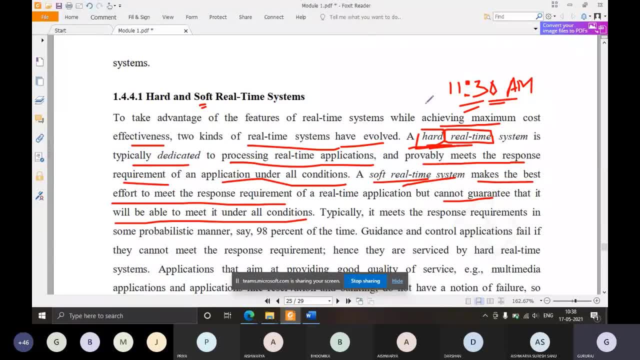 guarantee. So in such case say: late answer is still acceptable. That is what is the policy in soft real time system, And in soft real real time system, even though you you miss the deadlines occasionally, cannot every time. if you miss the deadlines. 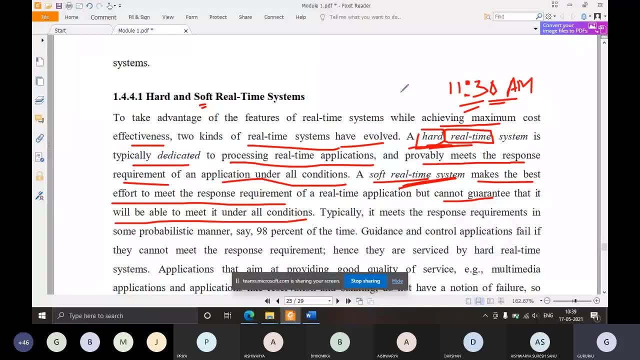 occasionally then it may not result in a unrecoverable or irrecoverable- you can say damage. Okay. so an example for software system is the ATM machine. okay so, from which, uh, the people will withdraw money. okay, so that is an example for a soft real. 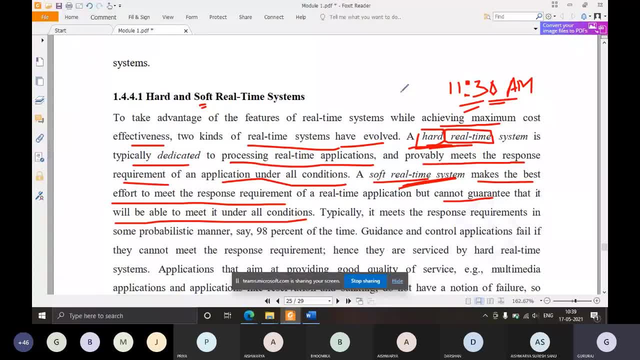 time system. so why? because, see, it depends on, uh, the network speed and these the state of the atm image. see, sometimes you can withdraw the money within five minutes because the system is very uh fast and the internet is very fast and the user is also fast, so he will input the required. 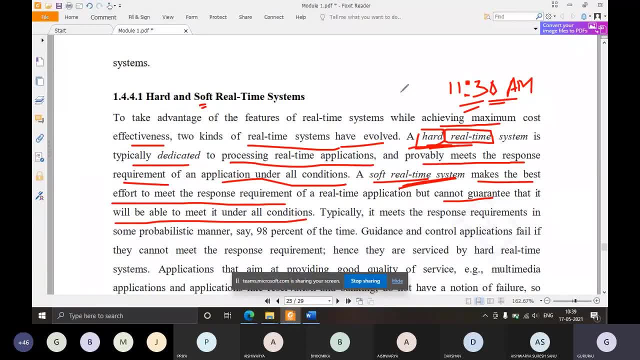 credentials properly and the money with, you can withdraw the money within five minutes. but the same system on some days. on some days, if you go and try to withdraw money, it will take 10 minutes to respond because it may be because of various reasons. it may be because of slow internet. 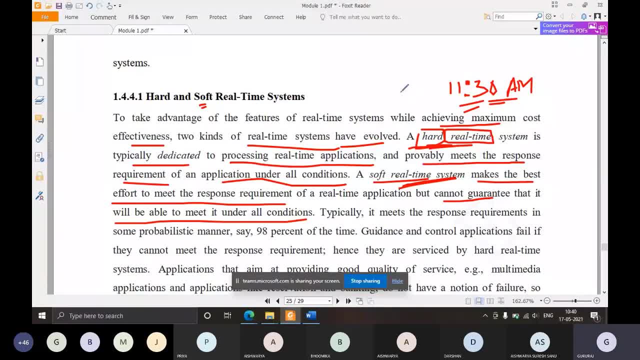 connection. it may be because of the health of the system. it is performing some updates, okay. in such cases, uh, the response of the system is slow for people, so in some days it will take 10 minutes. okay, so it depends. so maximum times it will not do any delays, but but on some occasions it may induce that extra time or extra delay, but that 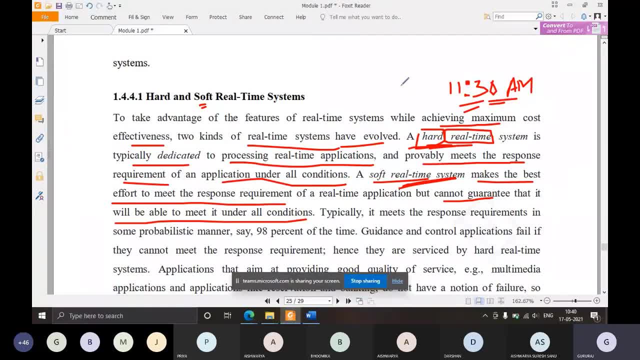 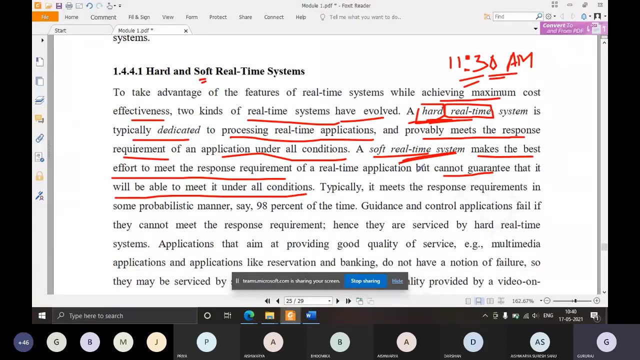 will not result in any unrecoverable damage. it will not result in any unrecoverable damage or output. okay, so what? what will happen? maximum is so the you can say: the person has to wait more, that's fine. so that is an example for soft real time application. 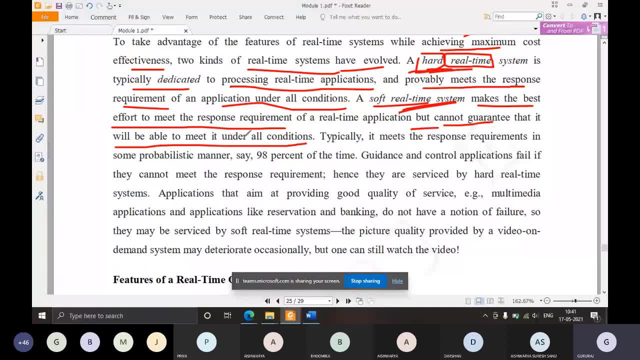 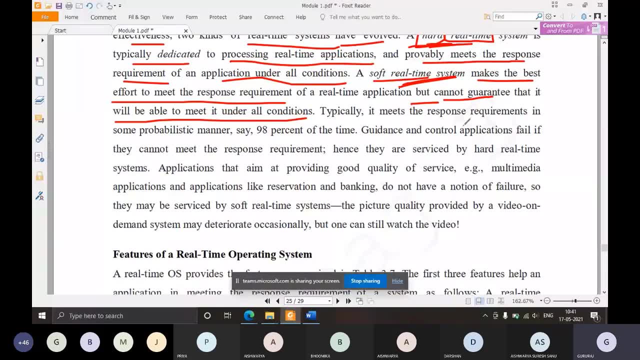 and so that is. it will put its best effort. but it cannot guarantee the uh that it will meet the deadline under all conditions. so typically it meets the response requirement uh for 98 of time, what is soft rate. so it will not miss the deadline every time. occasionally it will, it may miss. 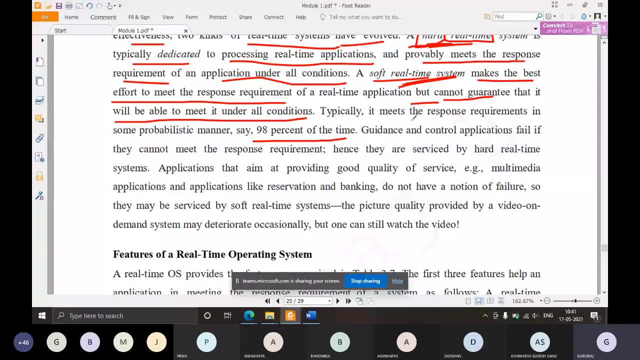 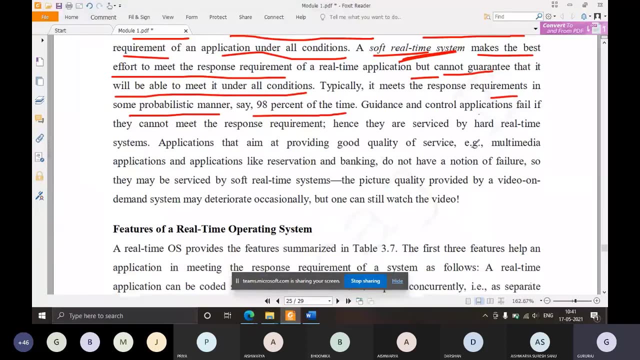 but even though that deadline is missed, it will not result in a irrecoverable damage. it will not result in a irrecoverable damage, so it meets the response requirements in some probabilistic manner. that is about 98 percent of time. so example for hard real time system is so guidance and 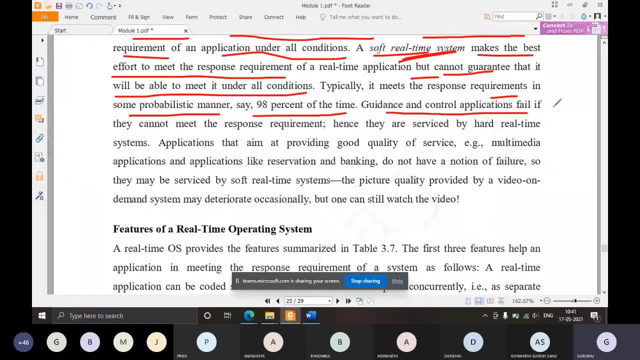 control application. if they fail? okay, if they fail by even a microsecond, so then they cannot meet the response requirement, since they come under hard real time system. and if they fail for even one microsecond also, the result can be catastrophic. okay, so instead of hitting, let's say: uh some. 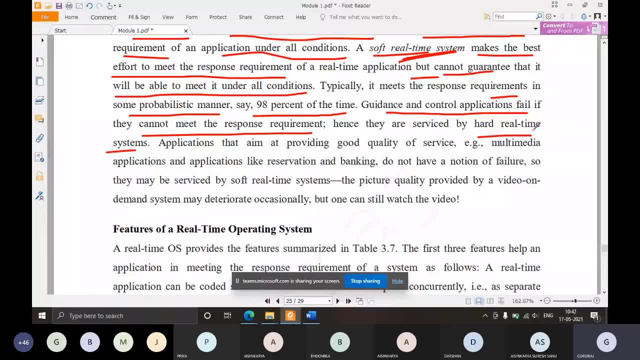 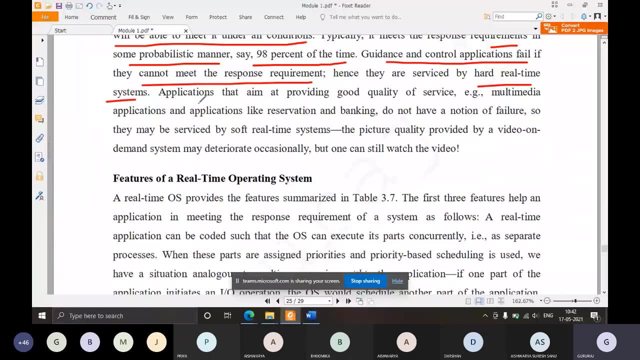 target, which is an enemy target. if, instead of the hitting the enemy target, it will hit the- uh, let's friendly target- okay, it will go and hit a friendly target- then the result will be catastrophic, okay. so some examples for soft real-time systems are multimedia applications and reservations. 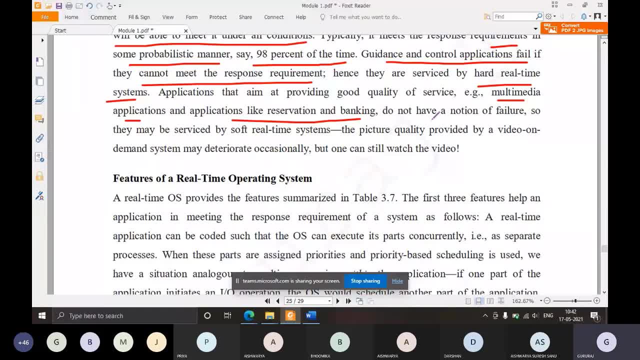 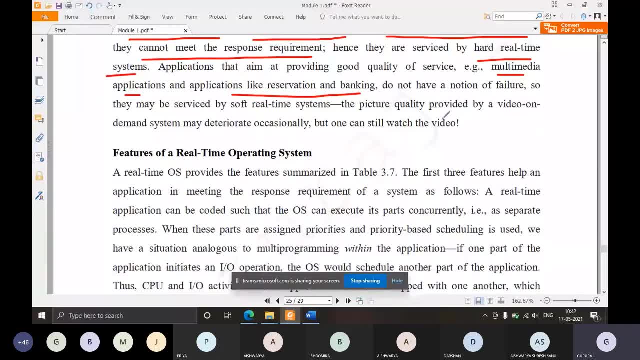 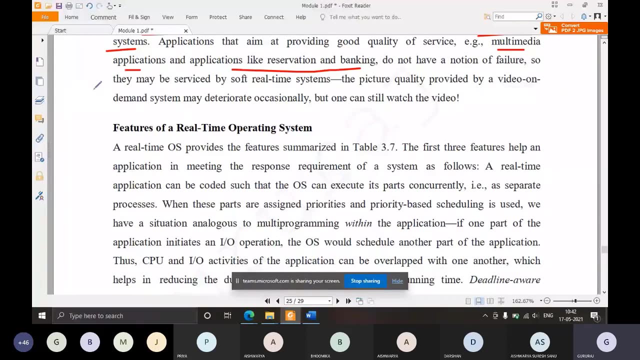 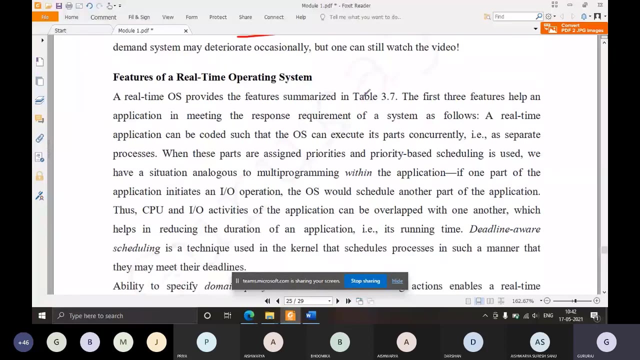 and banking systems, okay, so there. so there might be some random delays introduced, okay, which which will increase the response time, which will make them to miss the deadline, but definitely the result will not be catastrophic. so that is, they will come under soft real-time systems, so features of real-time operating systems. so there is a table here, so just go through this table. so 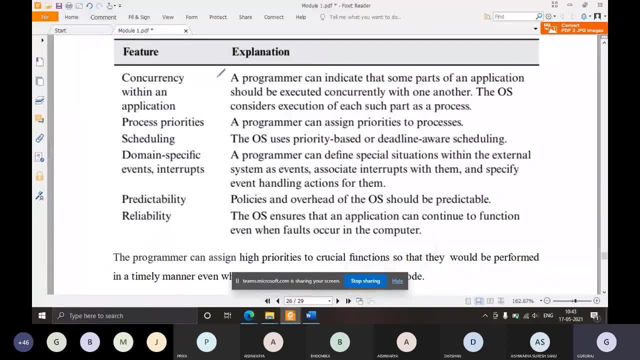 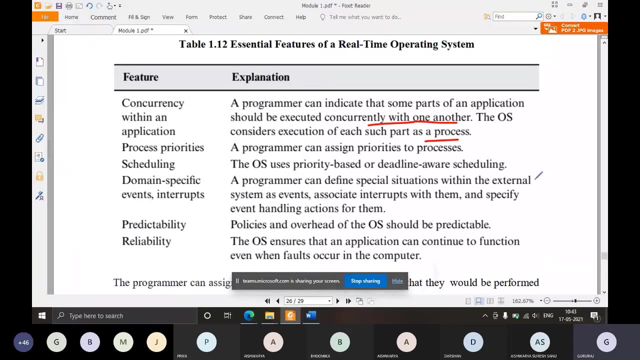 concurrency with an application. okay, so concurrency means so more than uh. one process is uh is being applied in one application. okay, so a programmer can indicate that some parts of an application should be executed concurrently with one another another. okay, otherwise considers execution of each such part as a process. see, till now we talked about execution of a program. okay, so execution. 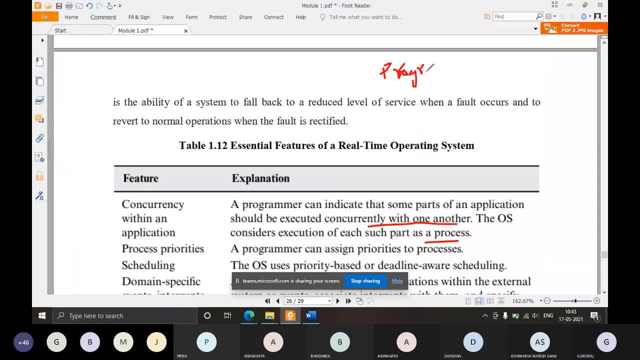 of a program, so usually as the systems evolved. so then what happened was a program or application. so a program or application will have multiple executions. okay, so each program will not have only one execution, but it will have multiple executions in form of what are known as processes. so they are known as processes. 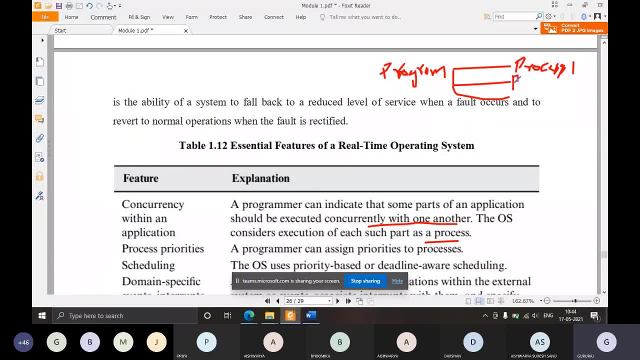 or process. so process one here, this is process two and this is processed. see all these processes- p1, p2, p3- belong to the same program. okay, even though they belong to the same program. so there there are three processes. this program is divided into three processes and these three processes- they may 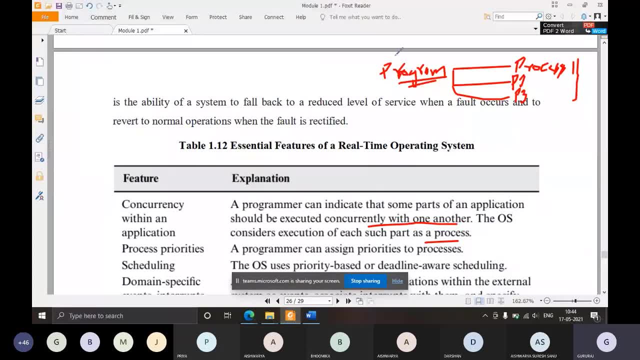 be executed simultaneously. okay, so that this execution of this particular program will be, we can say, uh, speed, speed up. so this, the application, the execution, will be faster. the execution of this program will be much faster. that is why it is split into three parts, known as process one, process two and process three, and you are executing all these three simultaneously. so 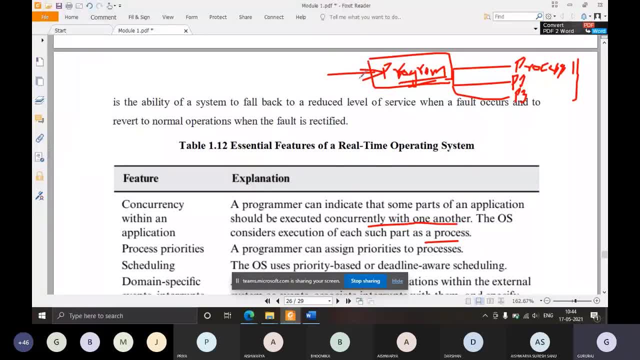 that the execution of this program will becomes faster will become fast. okay, that is the concept of concurrency within an application. fine. so this was not the case with previous operating systems. but as and when the operating system evolved, this concept came in, wherein you each program is executed or split into different parts, and all those parts are. 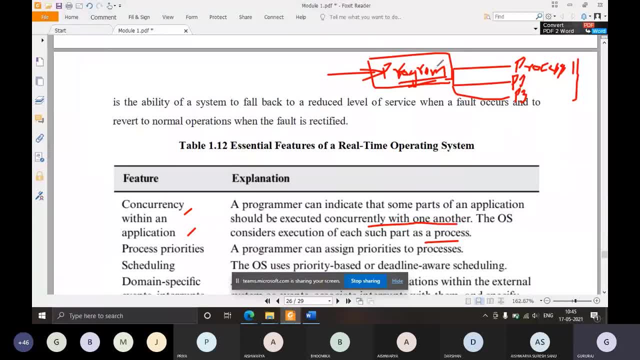 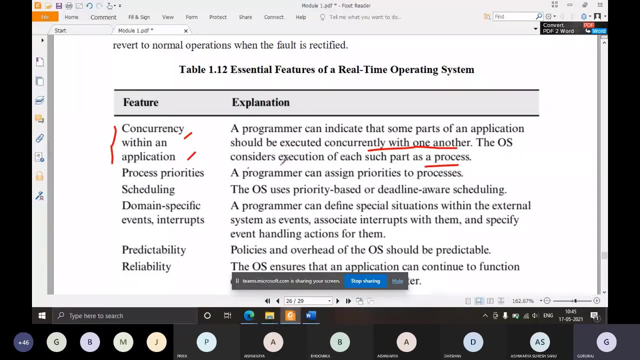 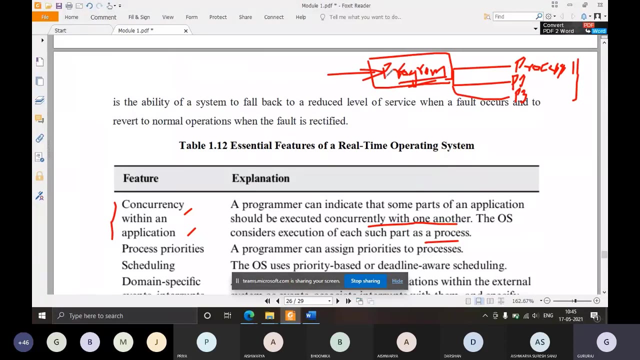 executed simultaneously so that the progress of the entire program it fastens up it. it will increase the overall execution speed increases. okay, so it is what is the first feature of real-time operating system? because you have to meet the deadline. so how will you meet the deadline? you have to execute the program fast. so how will you execute the program faster by? 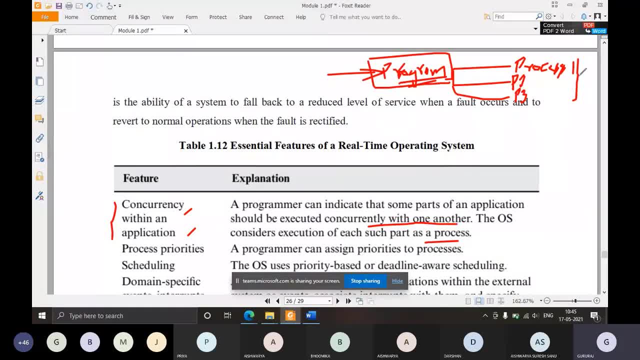 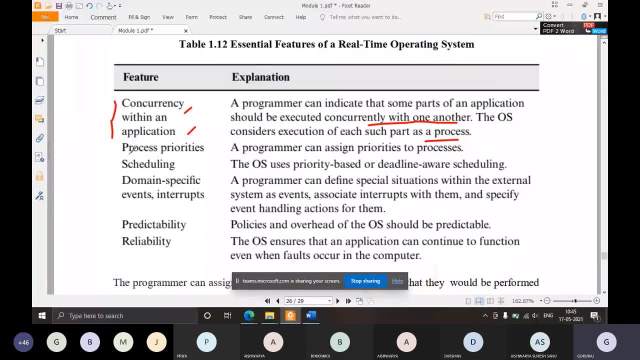 splitting the program into two or three parts and executing those two or three parts simultaneously. so it will speed up the program. so next feature is process priorities. so we have already seen this: process priorities are giving the process, the practice to each program or process. so this is 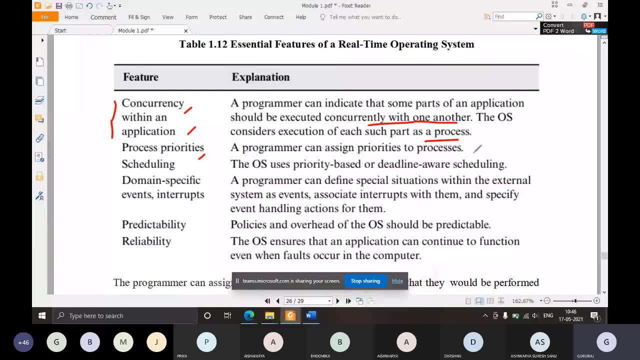 also already studied in multi-programming systems, multi-programming operating system, where in each process or program is given a priority. based on that, the scheduling will be done. so i have given an example of the teacher, hod and a principal. okay, so how their priorities vary and how they. 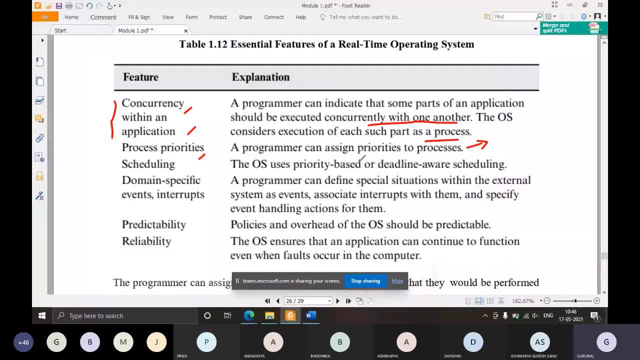 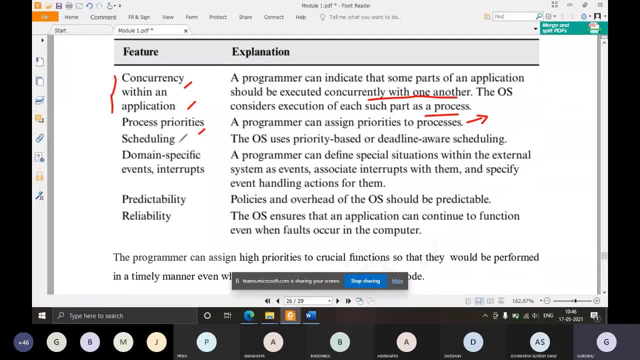 come and interrupt the lower priority program or process. that is what is process priority. this is the second feature for which will be available in real-time operating system with. with these concepts only you can achieve the deadline. otherwise you cannot achieve the deadlines or the you can say the response time. next is scheduling, so the os. 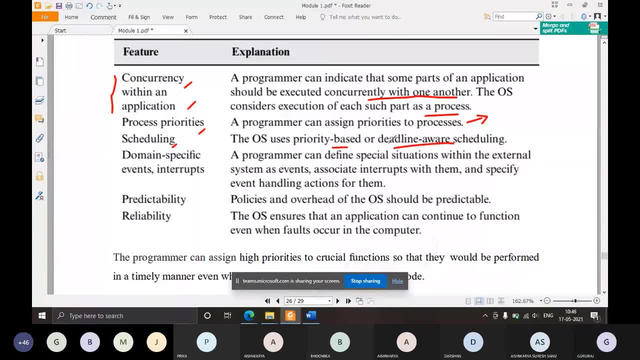 uses priority based or deadline aware scheduling. we already are familiar with priority based scheduling wherein if, let's say, if a program is being executed, is already in execution and if a higher priority program comes, then the present program will be paused and immediately the cpu will be assigned to the higher priority program. that is priority based. 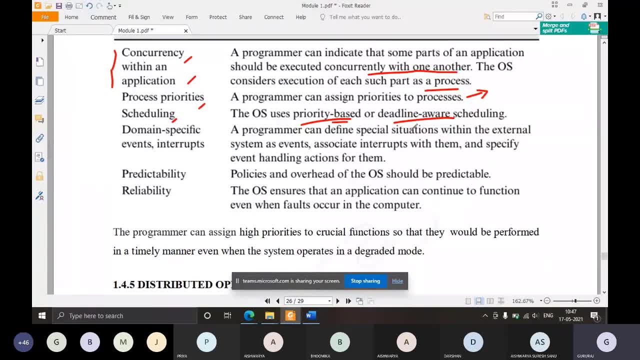 scheduling. so we are already available, aware of it. so next is deadline aware scheduling: see deadline aware scheduling means so as a, as we have discussed, so in real time of real time, applications will have deadline. so in in the previous example of storing the data from satellite, so the deadline was 1.99 milliseconds. okay, so based on this deadline, the scheduling. 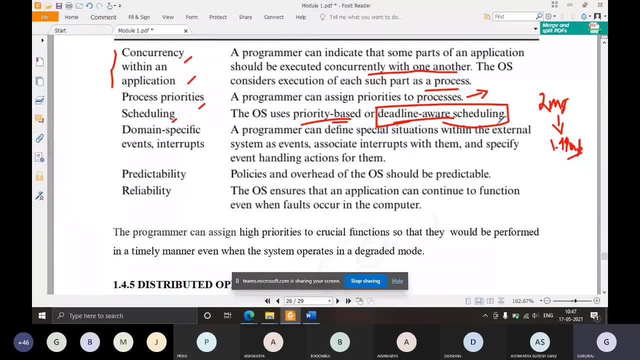 is done. so that is what is known as deadline aware scheduling. so the deadline was 1.99 milliseconds. deadline aware scheduling: see whichever process or program is having less deadline. okay, so let's say there is one more program which is having a deadline of 1.5 milliseconds. okay, so this program. 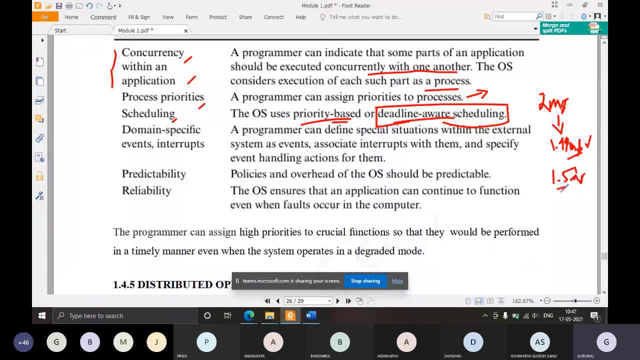 is having a deadline of 1.99 milliseconds, but this program is having a deadline of 1.5 milliseconds in such a case. so the program with a shorter deadline, the program with a shorter deadline, will be first scheduled. why? because it is having less time to complete itself, so it is given the chance for us to complete. 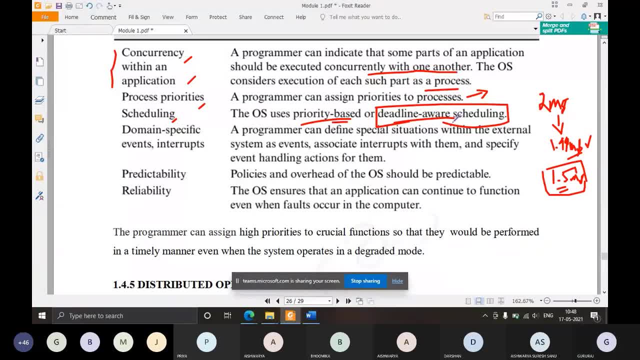 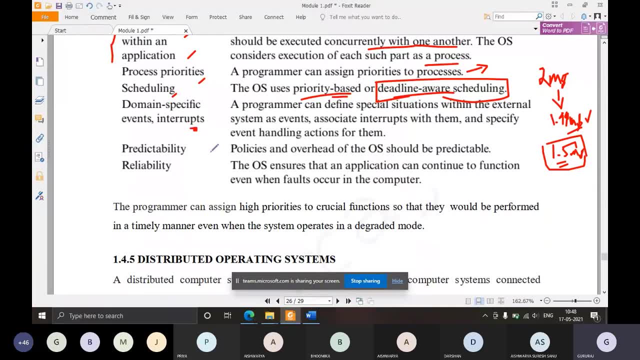 so that is what you mean by deadline aware scheduling. okay, so next is domain specific events interrupts: see in real time operating systems. what will happen is: each application demand is different. see an atm machine. application demand is different. a satellite guidance application demand is different, so a satellite guidance. 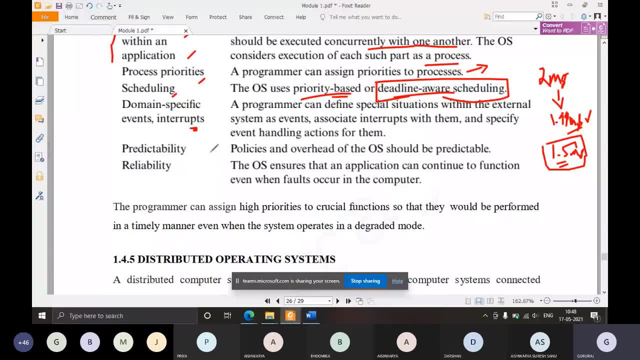 application may require the location data. okay, has to be updated every nanoseconds. but that is not the case with an atm application wherein there is no requirement of satellite data. okay, an atm machine need not know where it is placed. okay, it is not the requirement, so it does not want the 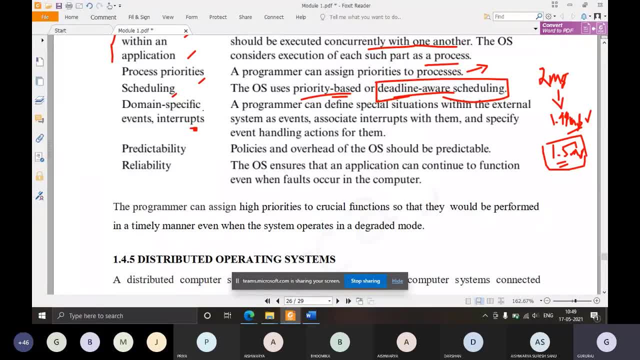 location service like that based on the application or domain. so each application demands a particular service. only such services will be included by the operating system. okay, so the real-time operating system for a atm machine is completely different from a real-time operating system for a missile guidance or a real-time operating system for a braking system. so those so the real-time operating. 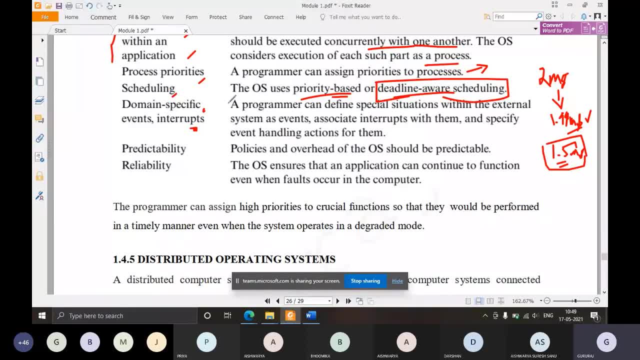 systems will be customized for every application, okay, and whatever the features are required for that application, only those only be will be included. okay, the example: in a for a atm machine, you may not uh require the uh the services for playing a song, okay, so there is no requirement. 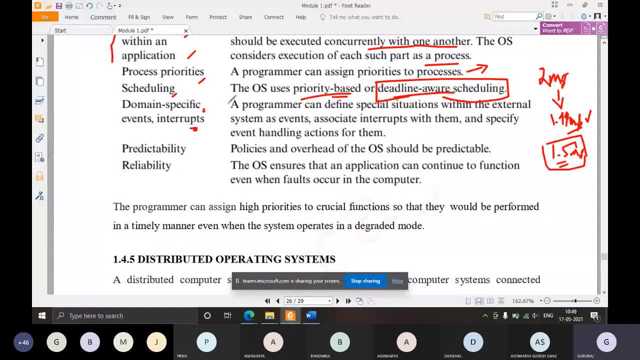 for apply for application in atm machine for playing a song. okay, so such, uh, such requirements, so such, you can say applications will be removed from the real-time operating system because for atm machine you need not, uh, you, you need not- play a song there. okay, so that service will be removed from the operating system. so by removing that service, 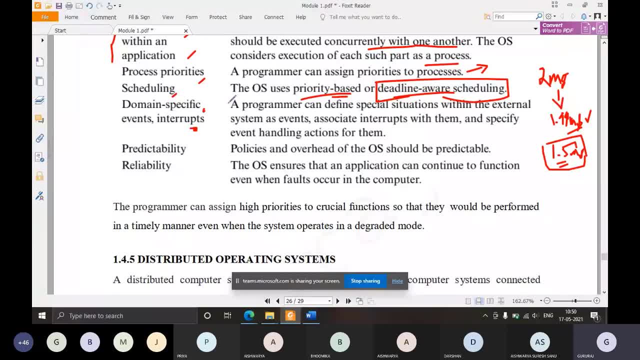 what you are doing is you are decreasing the space. one thing is you are decreasing the amount of memory that the operating system consumes to be stored first thing, and by removing that service you are improving the response time because you are reducing one service. if you are reducing one service, obviously the response time will go up. 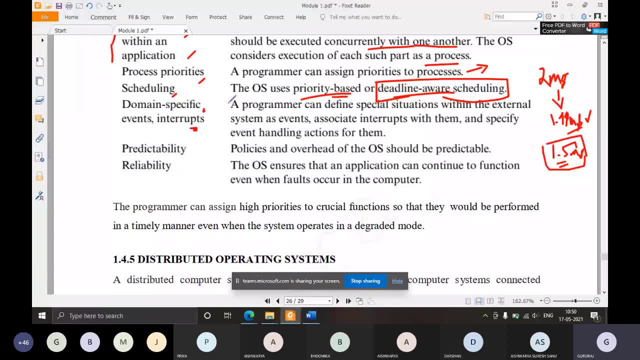 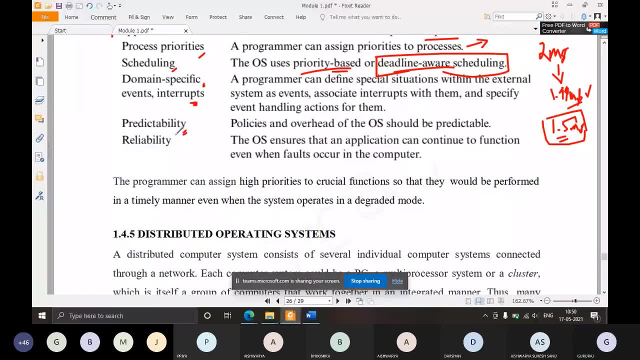 okay, so that is what: domain specific events and intraps. so next is predictability. this is very important. see, every time you you want to, let's say, do some job, the system should be predictable that it will complete the job by the so and so time. okay, example, if you want to play a song on your system. say i want to play a song through a loudspeaker, let us say play a session. i will play the té roman or a té format setting or olhať topography every day, for example, if you want to listen to your dépendouțe on the time of the day er pelarde- helpful to remember. if you are reducing one service, of course, obviously the response time will go up. 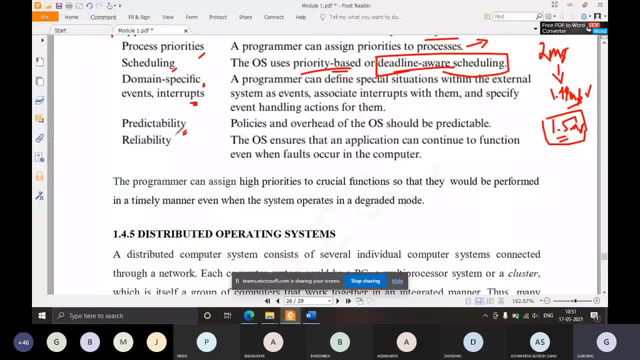 So every time you double click on a particular song, let's say, that song starts to play within 2 milliseconds, Within 2 milliseconds. whenever you try to open that song, it will open within 2 milliseconds. That is what you mean by predictability. 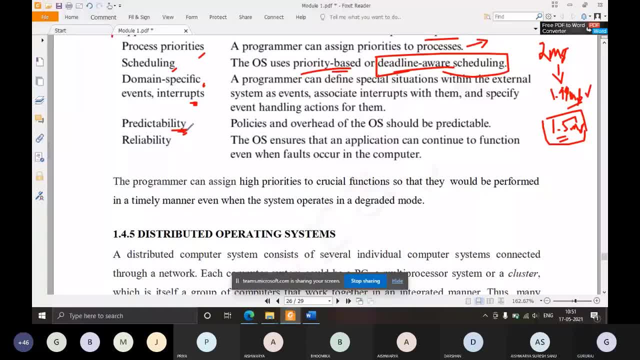 Policies and overhead of OSS should be predictable. Every time you open that application, it should respond within a particular time. That is what you mean by predictability. Next is reliability. The OSS ensures that application can continue to function even when faults occur in the component. 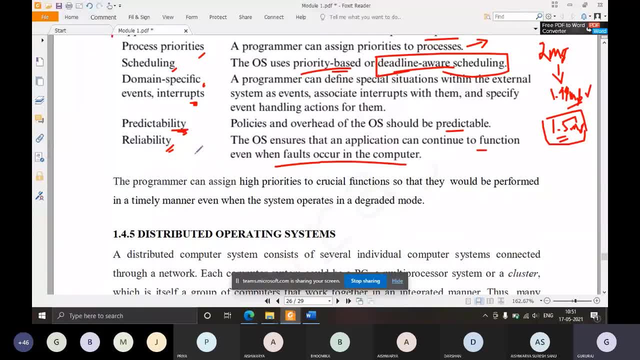 This is one of the extra techniques used here: Reliability- It is just like having a backup plan. That is what you mean by reliability. Example is: whenever you go for exams, You go for attending the exams. What you do is you carry two pens. 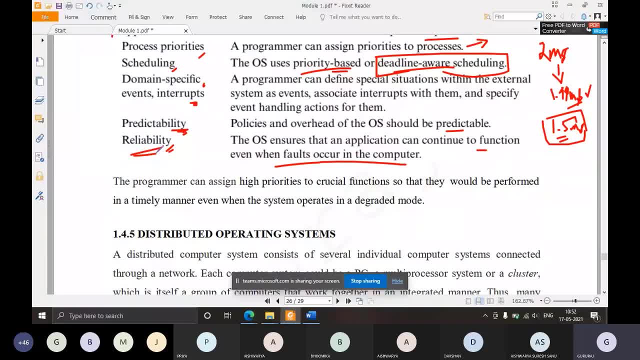 You carry two pens. If, in case, one pen fails, if it fails to write, there is always a backup. You can go to the second pen and you can still write the exam, Even though there is a fault that takes place in the system. 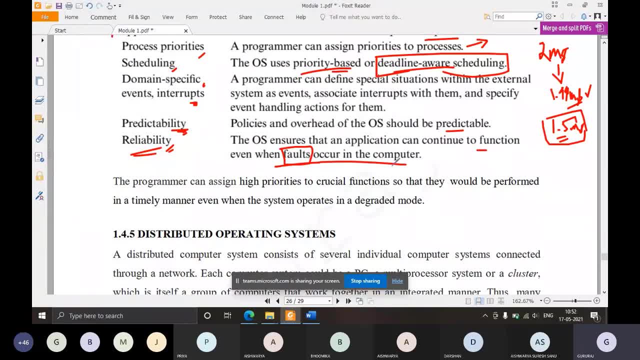 Fault means one pen does not work. Then there is a backup plan wherein you can immediately switch to the second pen And still you can continue your operation. You can still continue your operation or write the exam. That is what you mean by reliability. 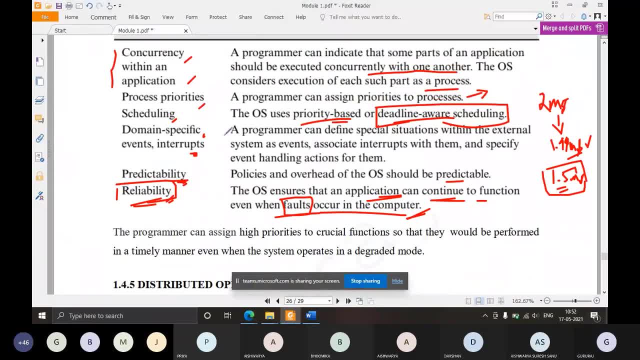 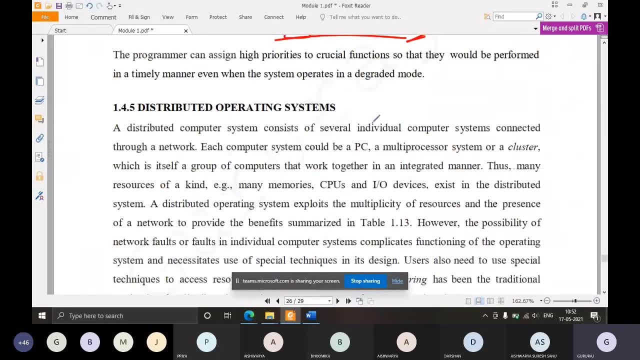 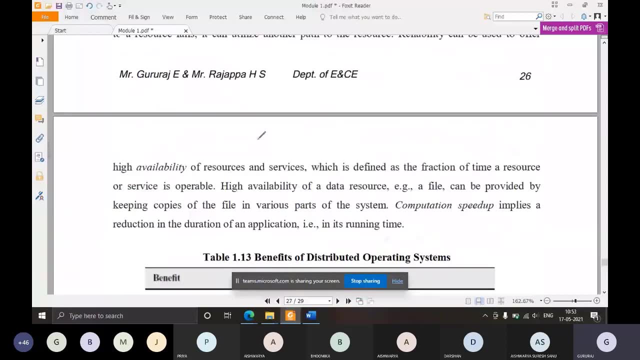 Improving the reliability. These are the features for real-time operating system. Next, the last class of operating system, the fifth one, is distributed operating system. As the name itself is indicating to you people, it is distributed means What will happen is. 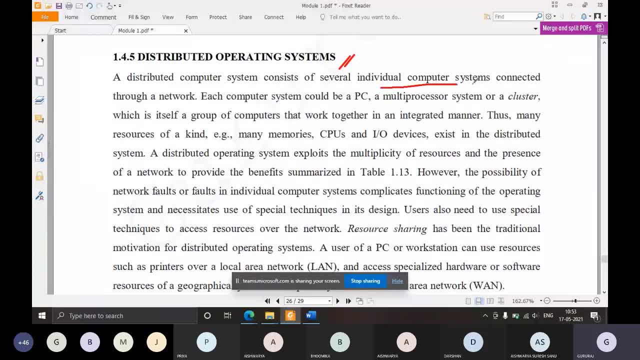 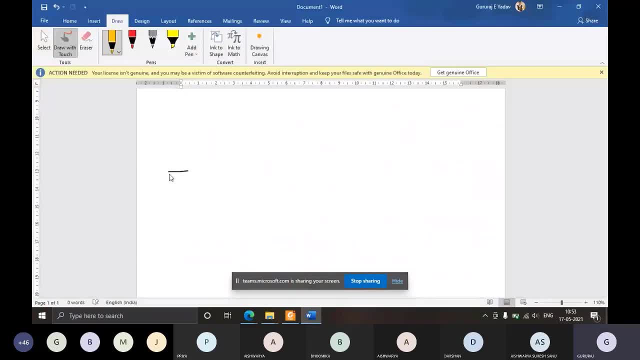 Distributed computing system. Distributed computer system consists of several individual computer systems connected through a network. So there are several individual systems connected through a network. So let us say: this is one computer, This is one more computer, This is one more computer And this is one more computer. 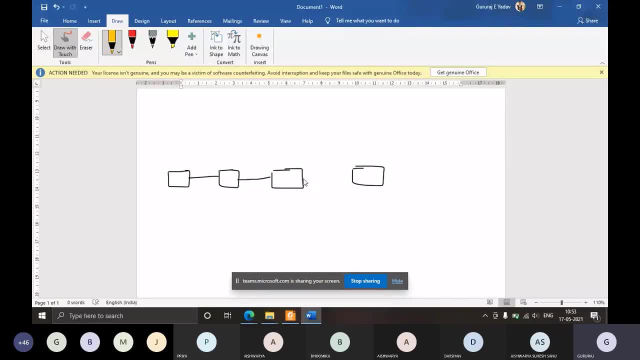 So all these four computers are connected through a network. So the network can be a local LAN network, Okay, So in wire or wireless network, anyone is possible, but they are connected with each other. Okay, You can see. this is the PC1.. 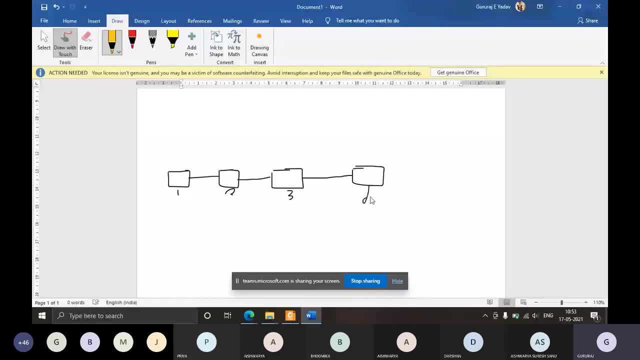 This is PC2.. This is PC3.. And this is PC4. And they are connected with each other. Okay, So this is what is the concept of distributed operating systems. And one more concept here is, let us say, this system, one PC1, has a printer known as P1. 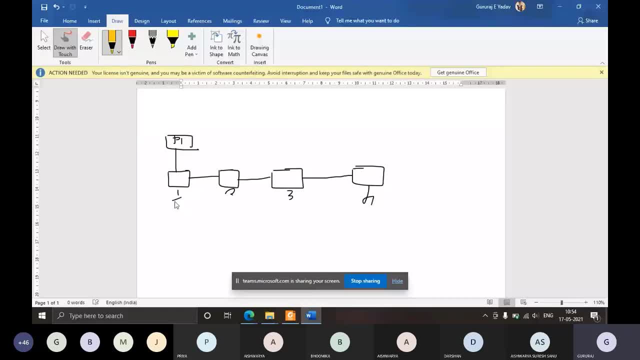 Okay, Okay, So this system, that is, PC1, is having the printer P1.. Okay, So now, since it is distributed control here, distributed control. so what will happen is if this PC4 wants to print something, okay, but it does not have a printer it wants to. 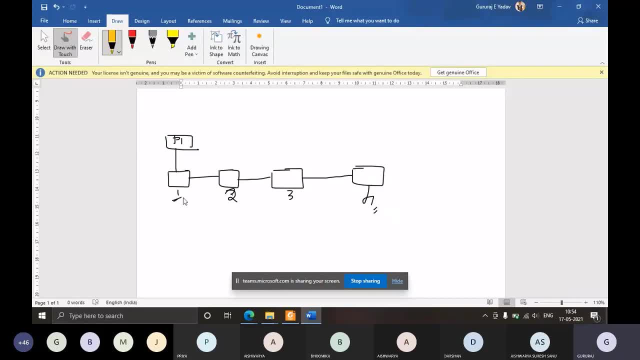 print a document but it does not have a paper. but since it is distributed control and they are connected with each other, So this PC4 can make use of this printer P1, which is connected to PC1. And it can do the printing. 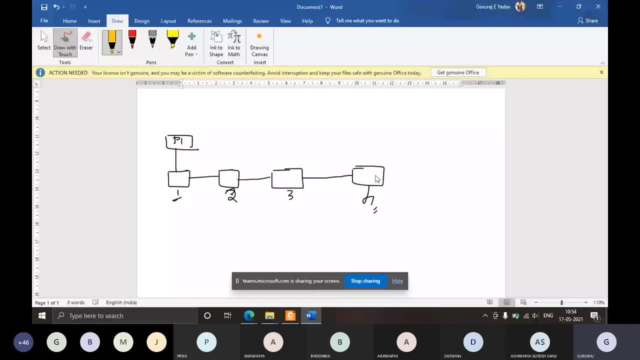 Okay, Since they are connected with each other. so the command given by PC4 will be sent to PC3, then PC2, then PC1, and then it will be sent to the printer so that the document will be printed. Okay. 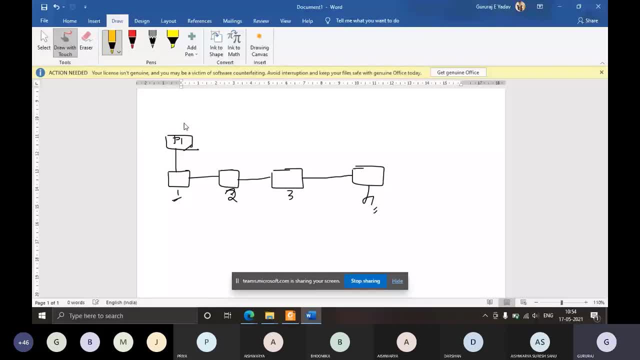 So it is known as: so this is what is the advantage, or one more feature of distributed operating systems. Okay, And one more thing, One more feature of distributed operating systems. Supposed this PC1 is given a job. okay, so let's say that there is a job, J1 that is assigned. 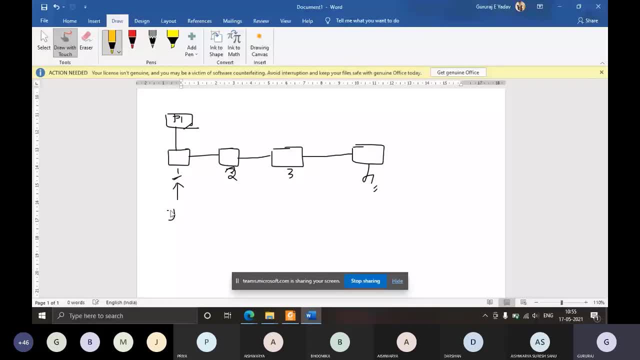 to PC1.. So this PC1 has to complete this job. Okay, So then what will happen is, since it is distributed control or distributed operating system, this J1, job J1 will be distributed among system 1, system 2, system 3, as well as system 4.. 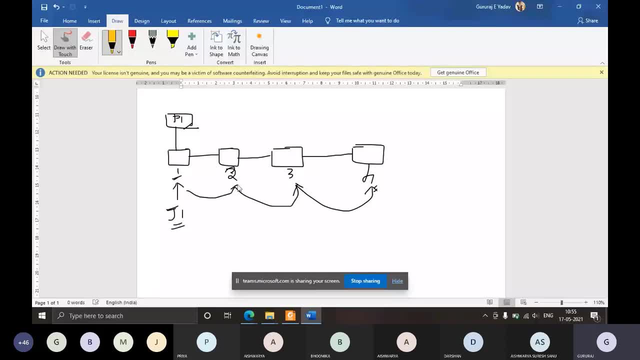 So the job is distributed. Okay, So the job is distributed to all the systems in the, you can say- network. So then what will happen is: this job will be completed faster. This will be completed faster. So how it will be completed faster. 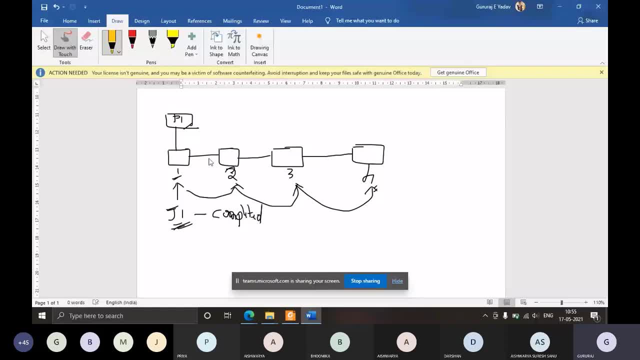 See if it is. if this job will be done by only one PC, obviously it will take more time. Okay, Now, what we are doing is we are splitting this job, okay, so that it is distributed to all the systems in the network. 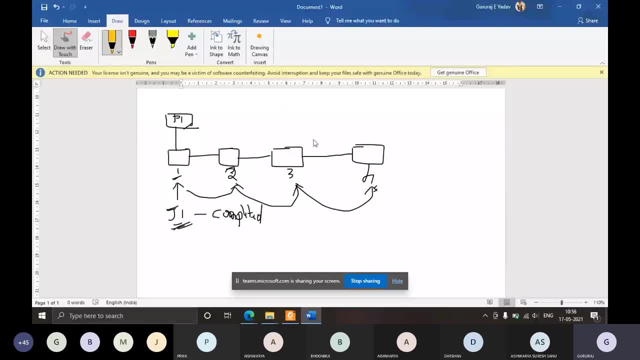 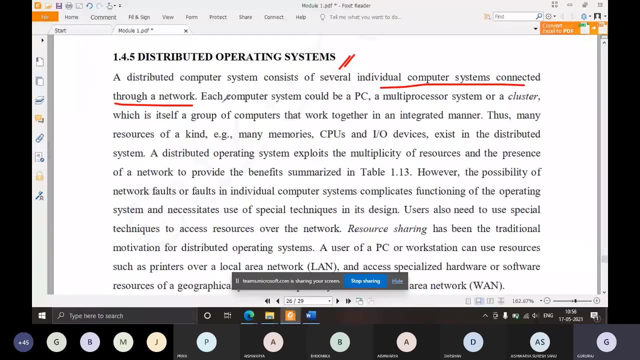 So then what will happen? Okay, So what will happen is all the systems will help to complete this job, and they do this simultaneously, So obviously, this job will be completed much faster. This is one more feature of distributed operating system. Okay, So each computer system could be a PC, a multiprocessor system or a cluster. okay, which is itself. 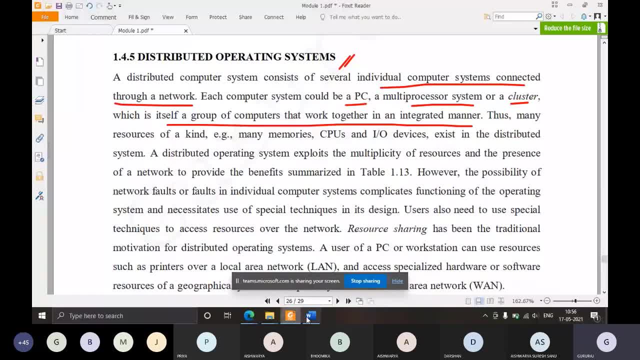 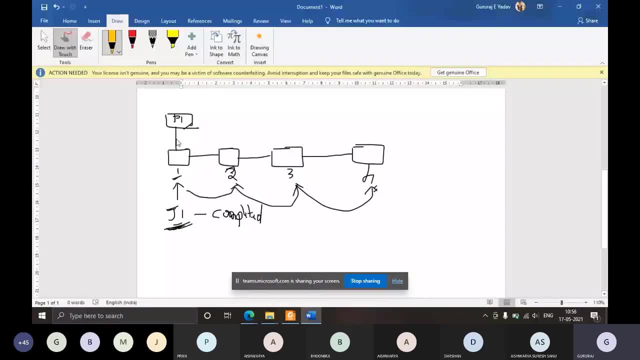 a group of computers that work together in an integrated manner. So same thing, whatever I told. So here this, this PC, this one PC can be an individual PC, or it can be a laptop, or it can be a microprocessor system, or this can be again a distributed operating system- distributed. 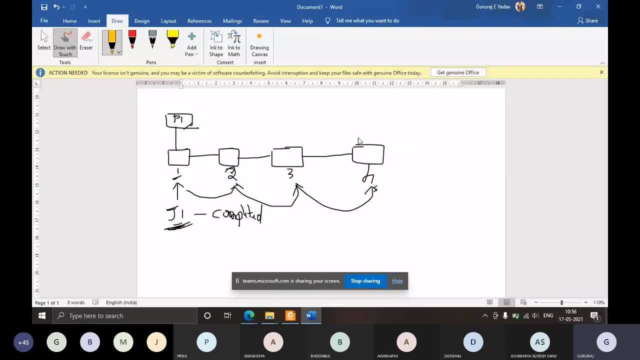 computer system. So this one system, one, or let's say this four system four, it may again have two or three systems. So these systems are called as 4-1, 4-2 and 4-3.. Okay, Okay. 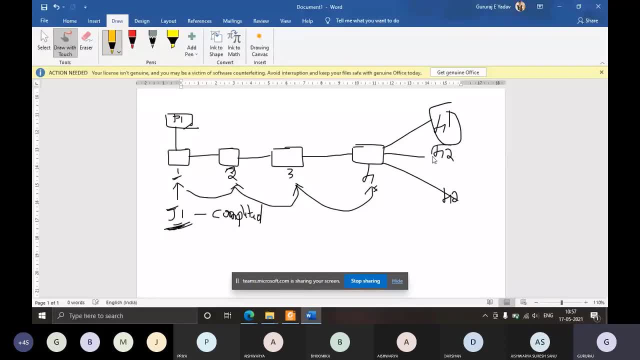 So what is this? So 4-1, 4-2, 4-3.. So system four is again nothing, but it's a distributed system, So which has three systems again, So one, two, three Like that. Okay, So that is what he says. So thus many resources of a kind example, many memories, CPUs and IOD devices exist in the distributed operating system, or distributed system. That is correct. So why? Because, see, there are four systems here and this fourth one is having again three systems. 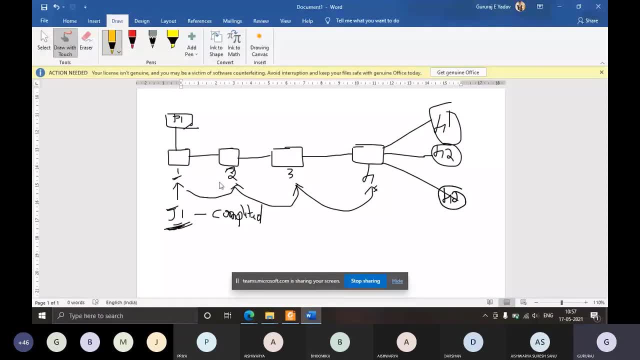 So, totally, there are one, two, three, four, five, six, six systems in here in this particular network, in this particular distributed system, and each system may have a CPU right. So this will have one CPU, this will have one CPU, this will have one CPU and this will. 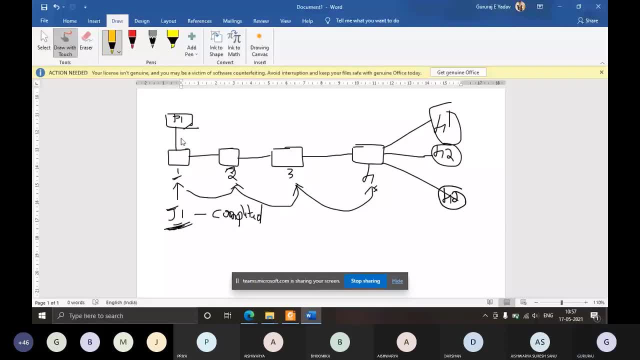 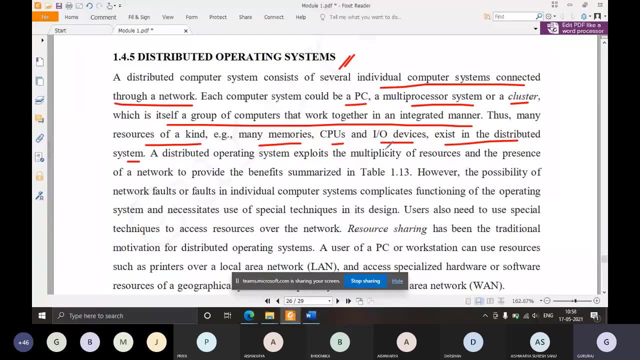 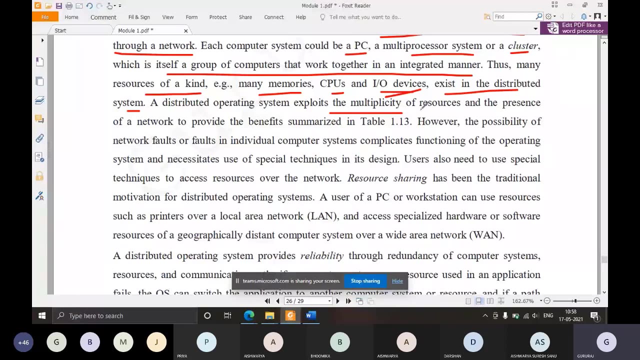 also have one CPU and these two will have again one CPU. So totally six CPUs, six separate memories- Okay. Six separate IOD devices like printers will may be existing, Okay. So distributing operating system exploits this multiplicity of resources. So this operating system exploits this property and what will happen is the presence of a network. 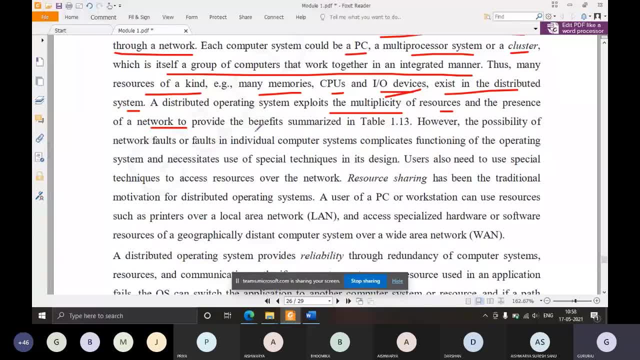 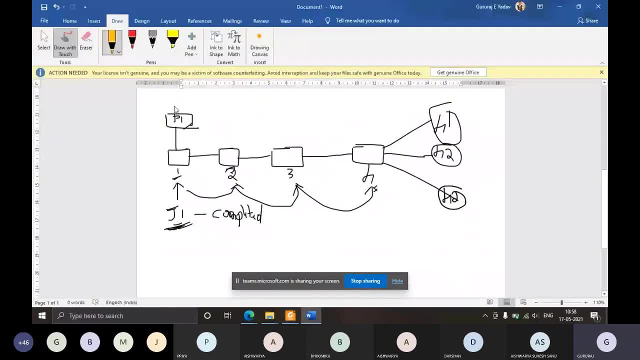 to provide benefits summarized in the following table. Okay, So what are the benefits? So, first thing is resource sharing. I explained that. So this printer, which is connected to the first PC, can be shared by the second PC, as well as the third PC, as well as the fourth PC. that is resource sharing. 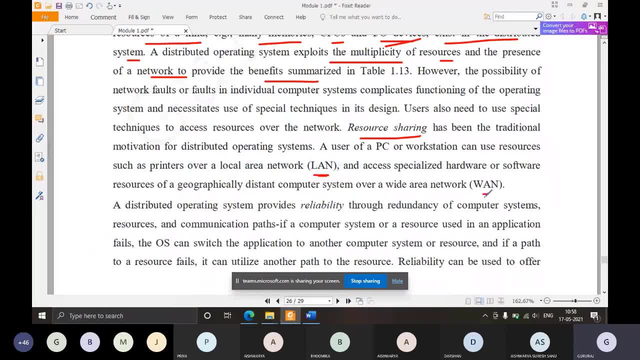 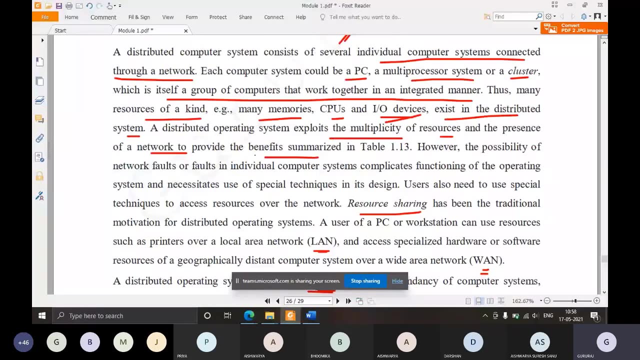 And this will happen through a local area network or a wide area network. So anything is possible. Okay, So next is distributed operating system also provides high reliability. So how this reliability is provided, see just now. we talked about the backup plan here. 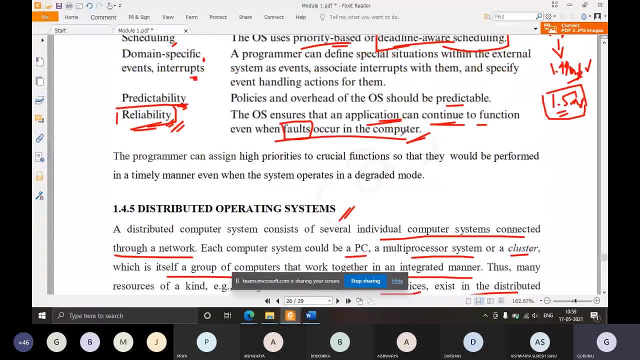 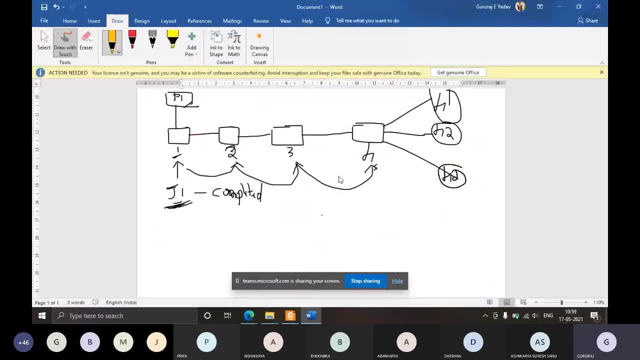 Okay. So if one pen fails to write, so you are having one more pen to use so that you can write the exam. Same thing will happen in distributed systems also. Okay. So what will happen is if, let's say, system four, if system four fails and it is doing. 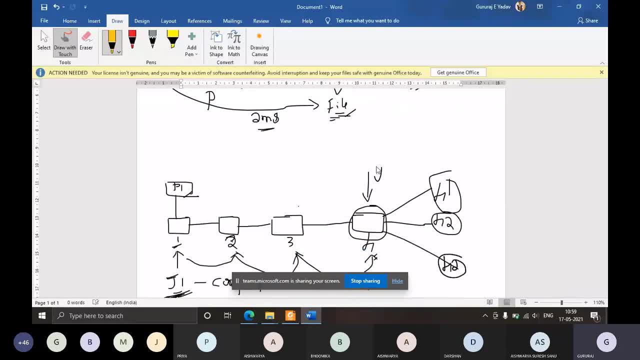 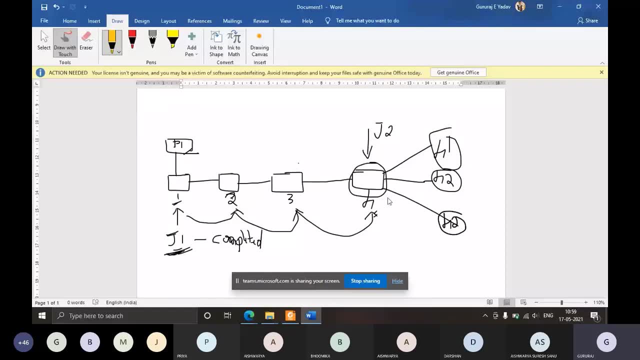 some job. let's say the job is J2.. Okay, Job is J2. and if the system four fails, then what will happen? There is always a backup plan, So that job J2 will be redirected. Okay To system three. 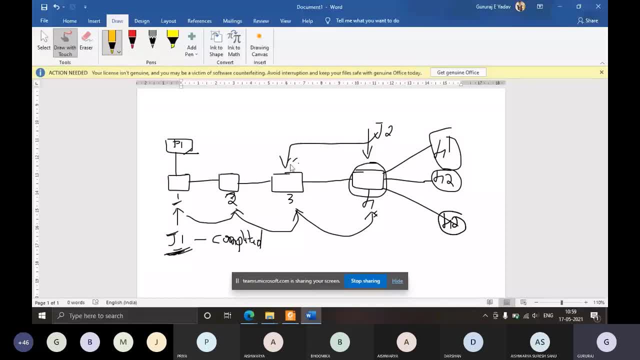 So, even though four has failed, the same job will be taken care by system three, because there are extra systems here in distributed systems. Okay, So same job will continue on system three. In the meanwhile, a system administrator will come and repair this system. four: 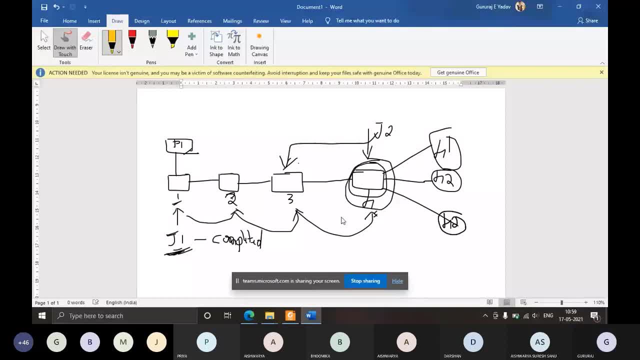 It is having some problem because it has failed. So some repair work can be done on this system four. Okay, In the meanwhile the operation will not be solved, So the same operation will be taken care by system three or system two or system one. 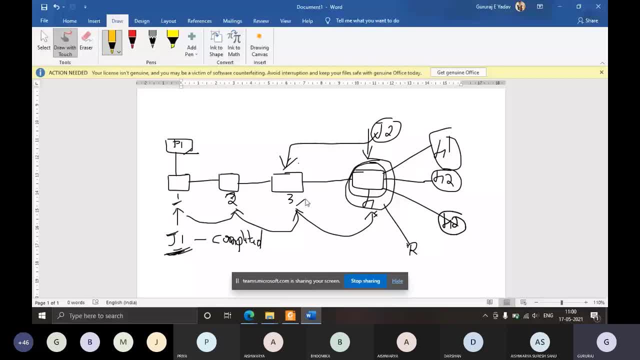 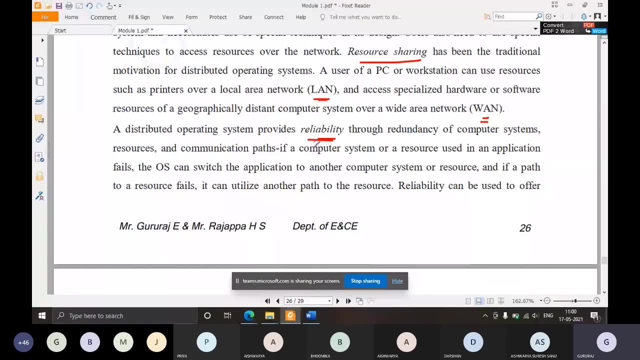 So this is the second you can say advantage of distribution, distributed control, Okay. Reliability, increased reliability, Okay. So see here, if a path to a resource fails, it can utilize another path to the resource, Okay. So next advantage is computational speedup. 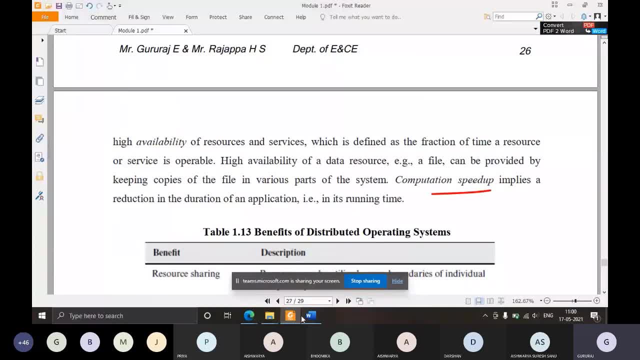 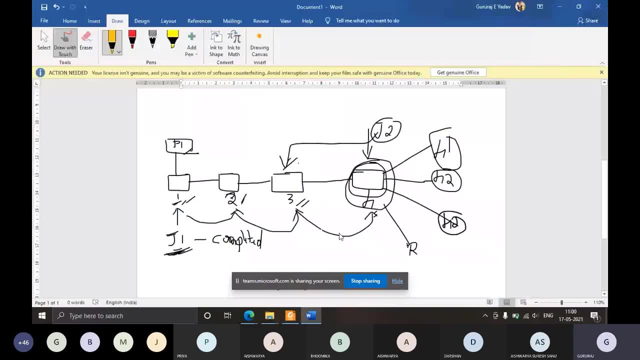 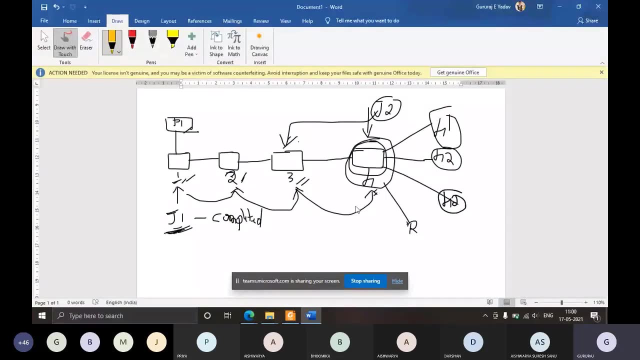 So that I discussed: Okay, So one job will be split into multiple jobs so that simultaneously it can be executed by all the systems in the distributed systems and it can be completed much faster. That is what is computational speedup. So same thing is discussed in the table. 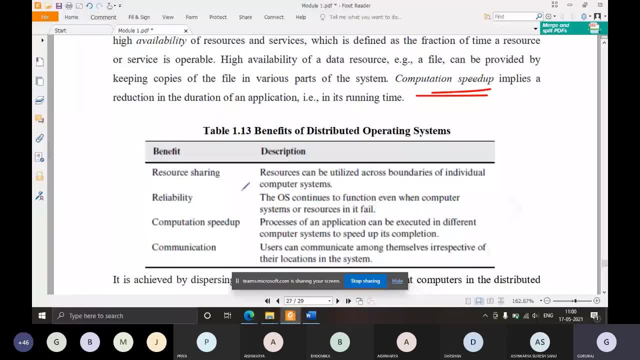 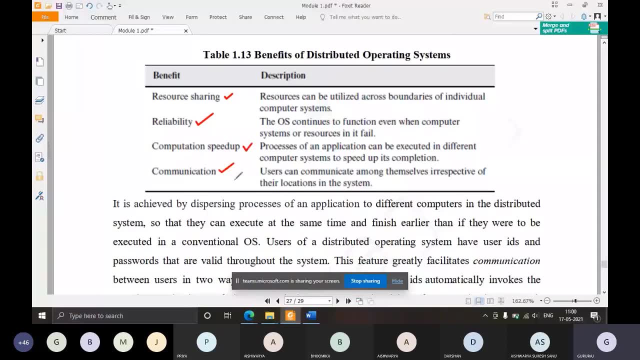 So one is resource sharing, next is reliability, speedup, computational and then communication. Users can communicate among themselves, irrespective of their locations in the system- Okay, You already know. using internet or through internet, So a person sitting in one country can communicate with another person who is sitting somewhere. 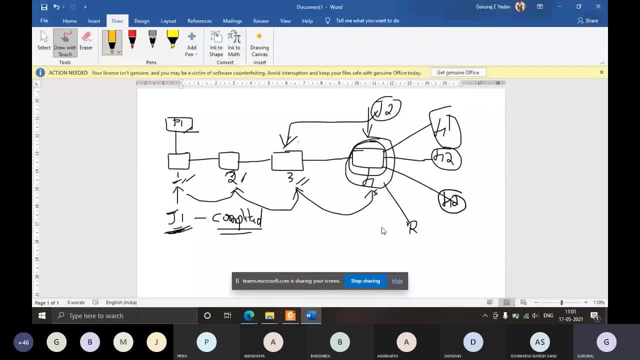 in the world. Okay, So one person is sitting in UK and one person is in India. They can still communicate, they can still do video calls, they can do voice chats. they can do simple chats, text chats also. this is possible. 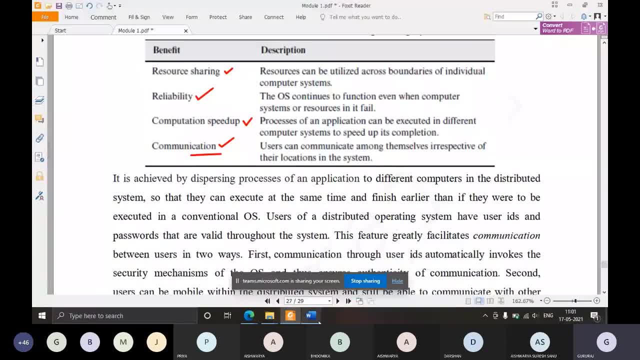 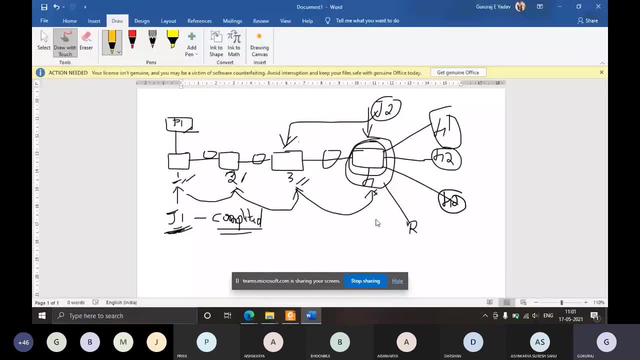 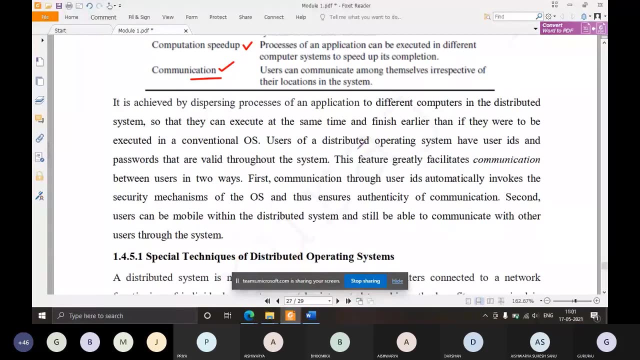 Okay, So communication First of all, they are connected, as this connection can be wired or wireless, So this can be LAN or a WiFi network. So that is available and it is optional. Okay, Next is special techniques of distributed operating system. 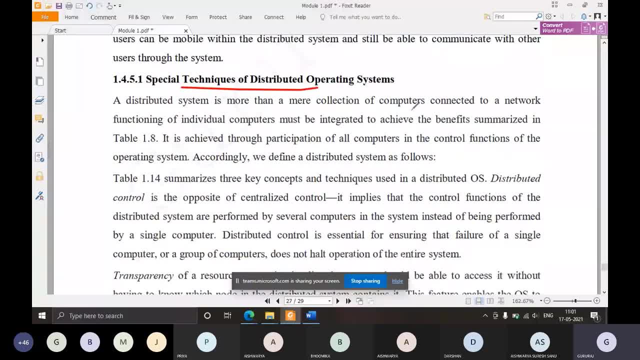 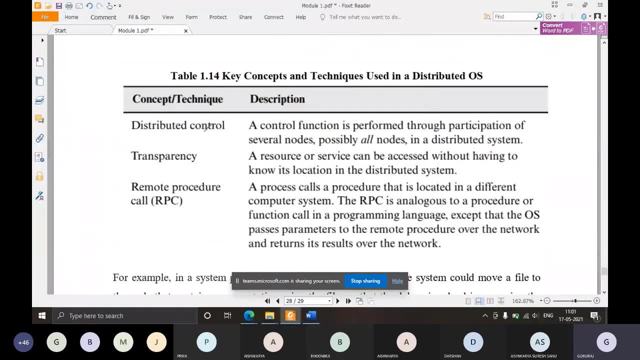 What are the some techniques that are employed by the distributed operating systems? Okay, So for this you can directly refer this table: distributed control. So a control function is performed through participation of several nodes, possibly all nodes, in distributed system. So that is what fitting this job. So a job is given. 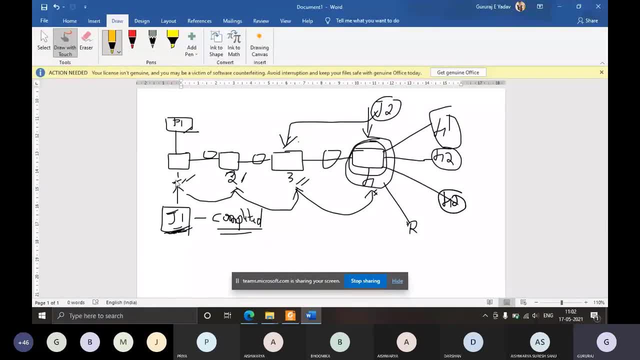 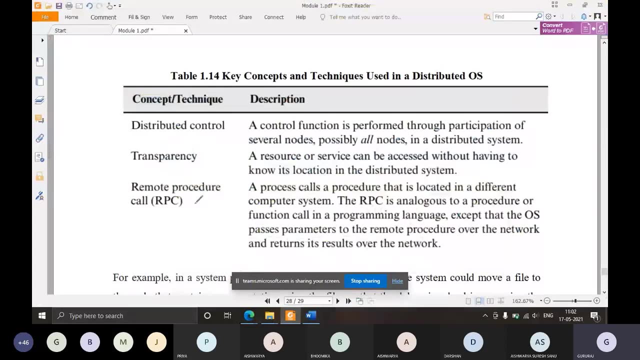 to PC1.. So PC1: what it will do is it will distribute the job to all the systems in the network So that all will work towards the completion of that particular job and it will be completed at a much faster rate. So that is what is distributed control. Next is transparency. 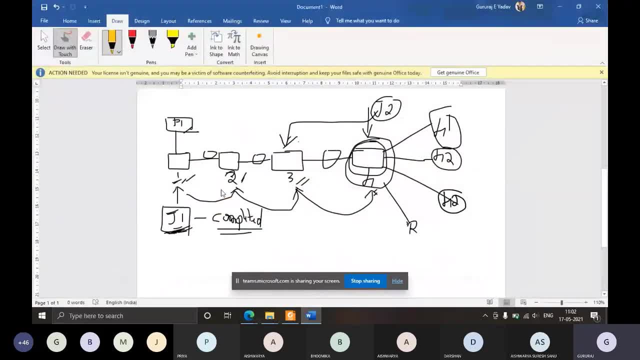 What do you mean by transparency? This printer, which is connected to PC1, it is transparent to all the systems. So this is transparent to system 2, it is transparent to system 3 and this printer is transparent to system 4 also. See, transparent means that resource can be available. 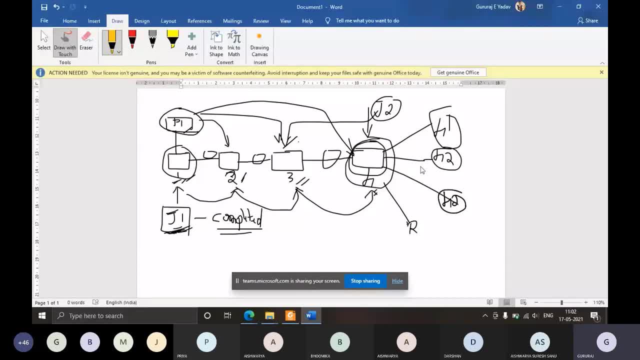 to all the systems. So this is transparent to system 3 and this printer is transparent to system 2.. It is available to all the systems that are in the distributed system network. In the network, whichever systems are there, it can make use of the resources and it is transparent. There is no. 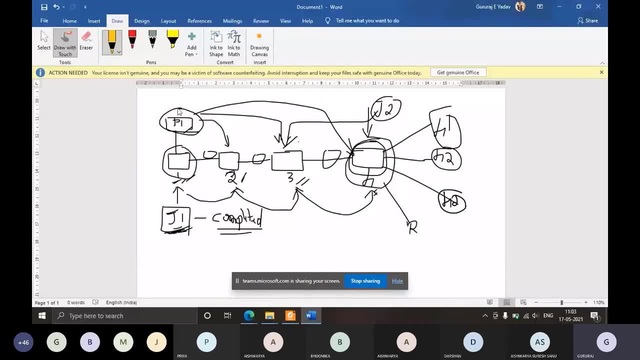 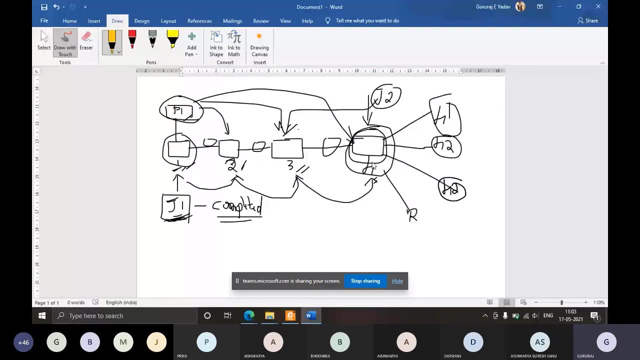 hiding here. So that means PC1 cannot hide the printer, saying that this printer is mine. no other can use this printer. That is not there. Transparency is there. So any resource available with any system is visible to all other systems in the distributed network of systems. Next is remote procedure call. 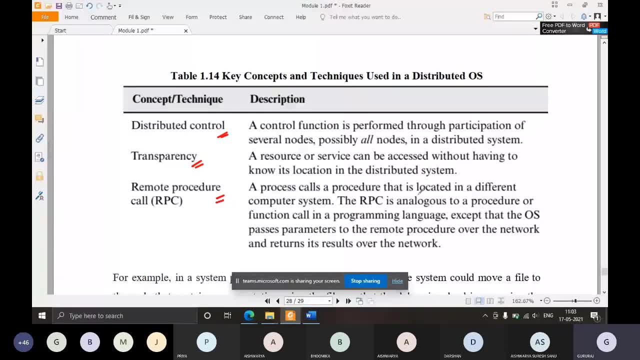 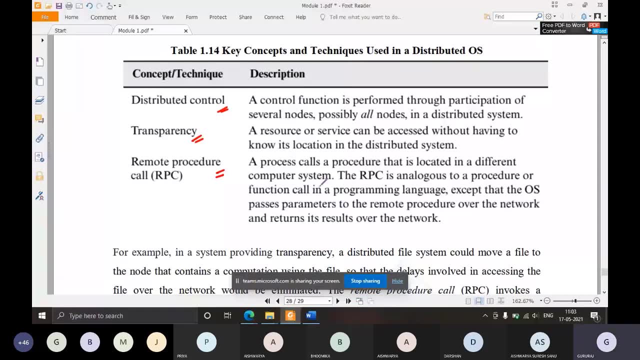 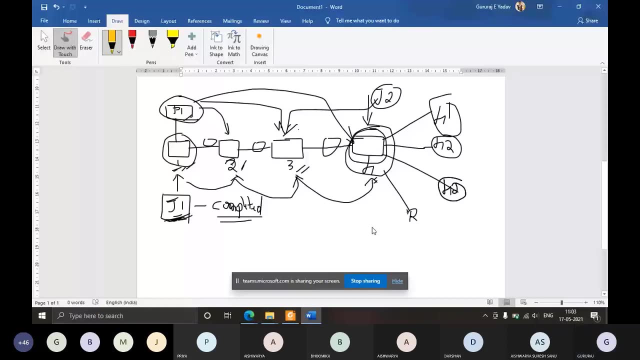 So the process calls the procedure that is located in different computer systems. What do you mean by that? is The example. Suppose system 4, this system. it has, let us say, the word application. It has the word application. Okay. 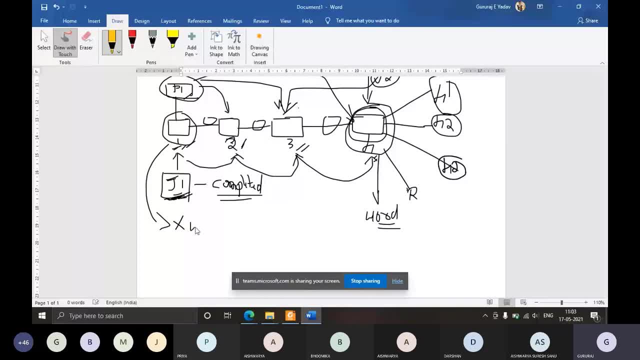 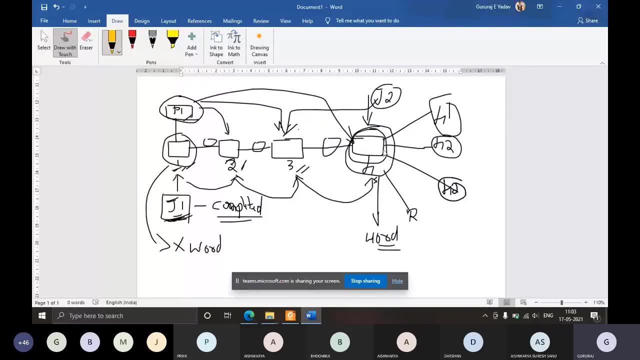 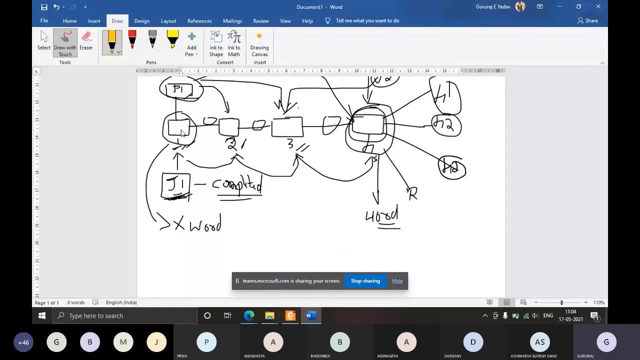 For system 1, it does not have the word application, It does not have word. Yeah, getting the concept, So Microsoft word. So Microsoft word is available in system 4, but it is not available in system 1.. So now there is a job given to system 1 which involves word application. So it will involve some data processing or text processing application using word. It has to open this word, but it does not have this application. 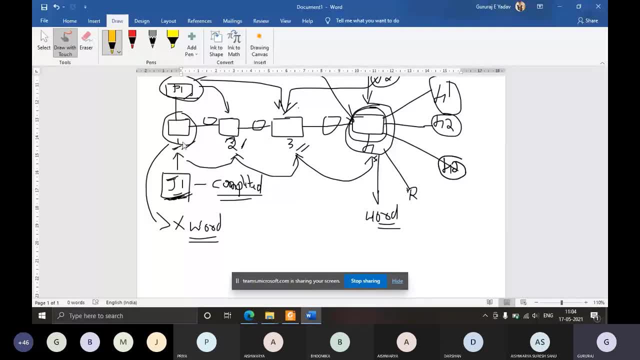 Okay, what it will have is what it will do is system one will invoke this application, this word application, which is in system 4, using what is known as remote procedure call. okay, using this function or option, it will. it will do this job. okay, so remotely, it will open this application. 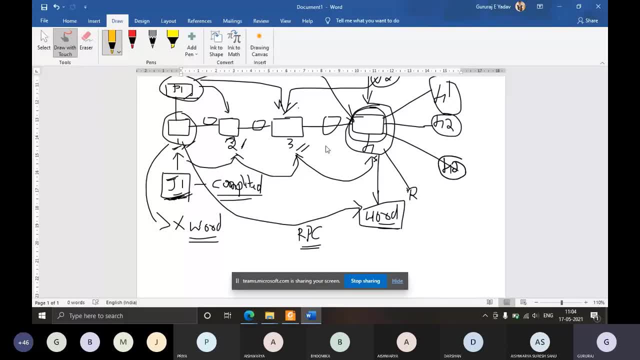 word application which is not there in this system but it is there in another system, in the same network, in the same distributed network. so this process is known as remote procedure. call some application or some program is there in another system and that program or application will be invoked, or it will be called by a system, by another system, but it is there in the same. 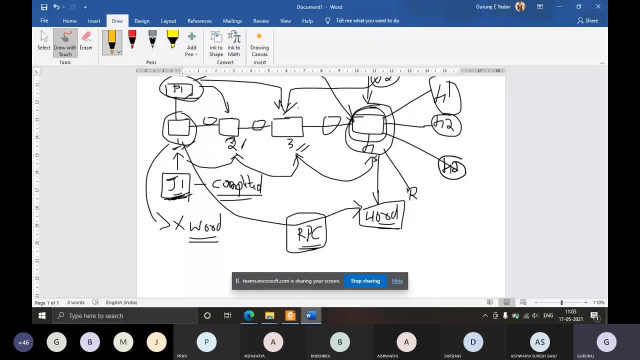 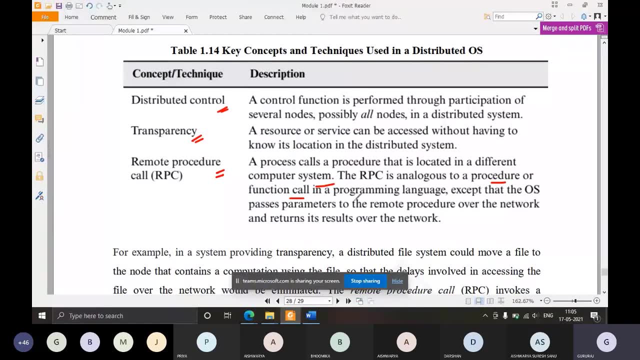 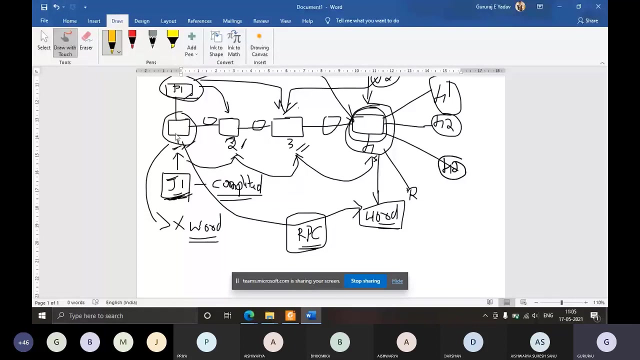 network. okay, that system is there in the same letter. so this is what you mean by remote procedure call. so it is analogous to procedure or function call in a programming language, except that the os passes parameters to remote procedure over the program and returns the results. okay, so it is not calling any function within the same system, but it is. it is calling a function. 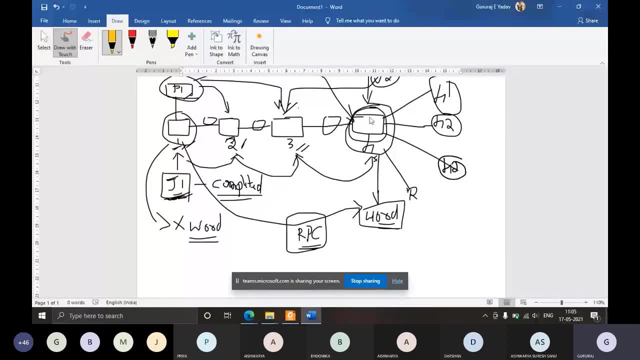 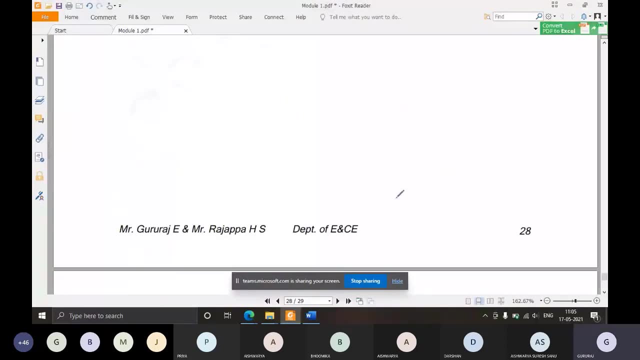 or a program that is available in some other system, but that system in this is is available in the same network. okay, that is what you mean by remote procedure call. that's all. okay, this is about the distributed operating systems. okay, so there are some recommended questions here. you can go through that. 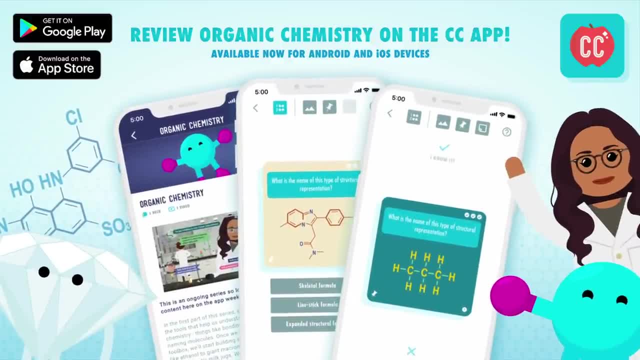 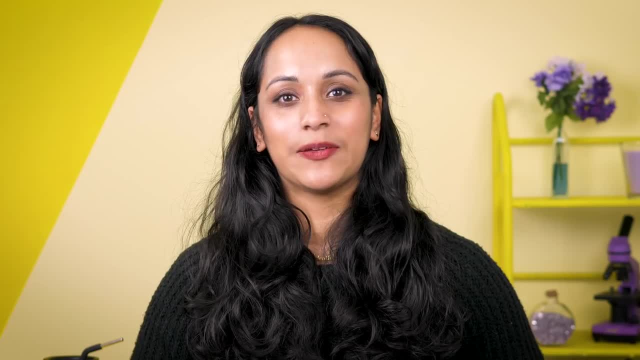 You can review content from Crash Course Organic Chemistry with the Crash Course app, available now for Android and iOS devices. Hi, I'm Deboki Chakravarti, and welcome to Crash Course Organic Chemistry. We've gathered a pretty impressive toolbox of chemical reactions. 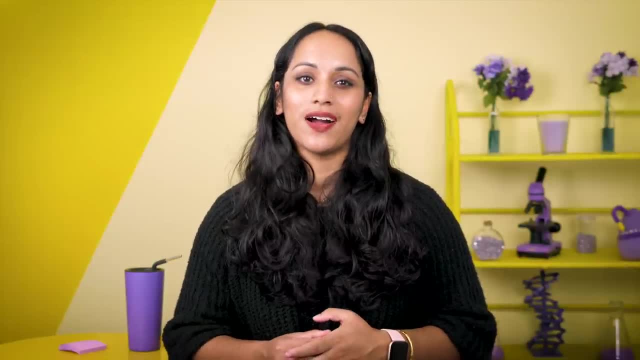 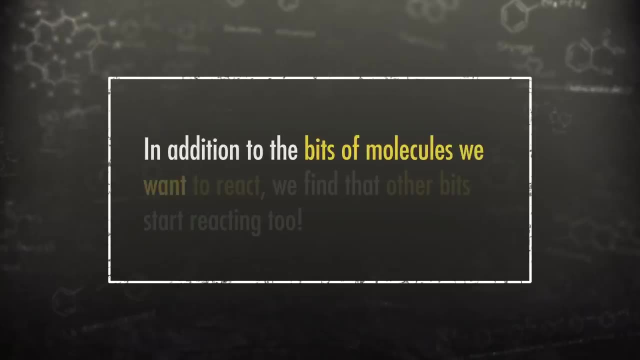 and can use them to transform a lot of functional groups we might come across. But as we meet more complex molecules we run into a problem. In addition to the bits of molecules we want to react, we find that other bits start reacting too. 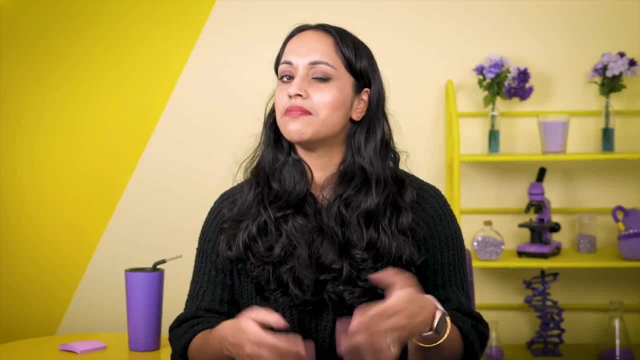 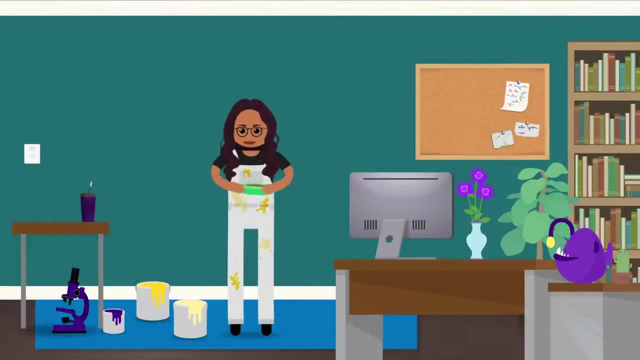 Imagine for a second: you're going to paint a room in your house Like, maybe purple and yellow, to turn your office into a remote set for Crash Course. If you're being careful, you'll use painter's tape to cover up the edges of window frames. 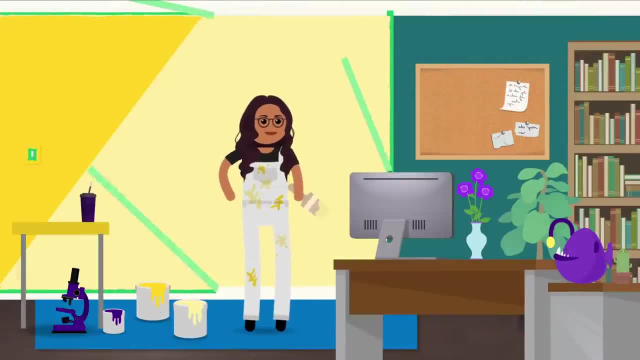 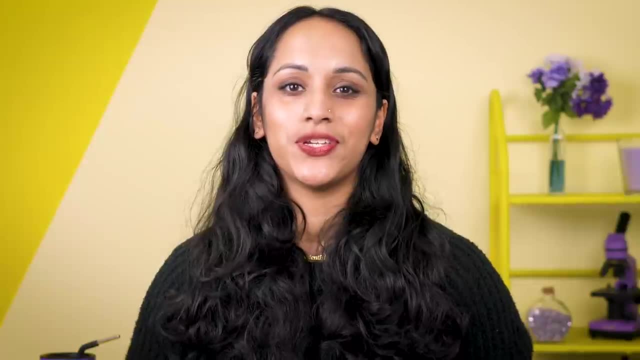 light switches or decorative trim. Once you've finished painting, you peel off the paint splatter tape, revealing those pristine old surfaces in your otherwise new room. And we can do this with molecules too. We can prevent a functional group from reacting by 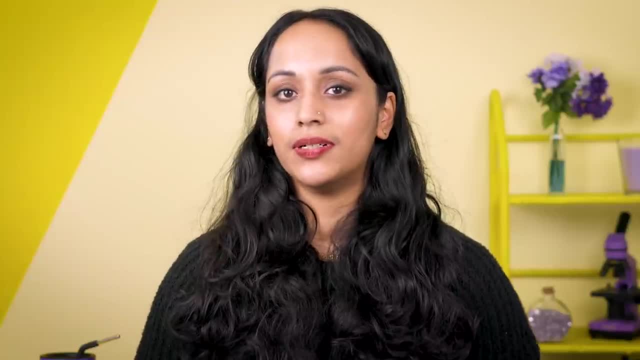 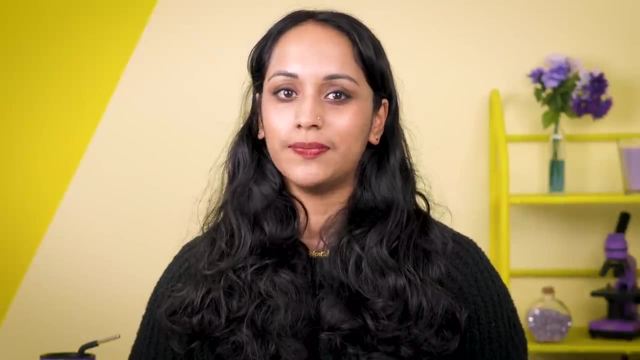 taping over it before we throw a bunch of reactants. Then we remove the tape at just the right moment. so our original functional group remains in the otherwise new molecule. This painter's tape for chemical reactions can go by many metaphorical names. 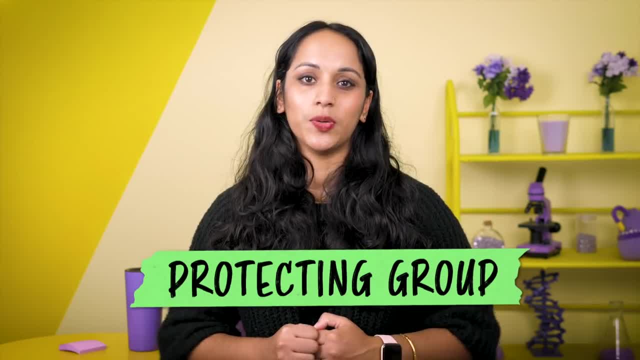 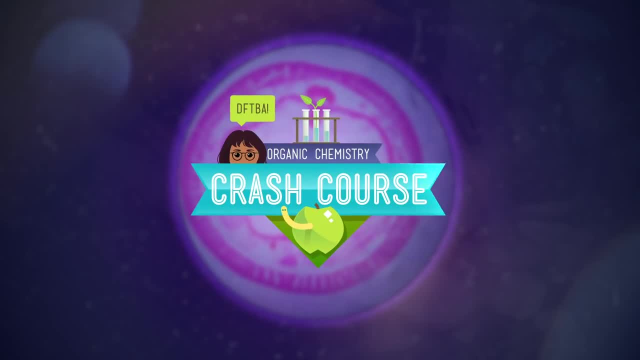 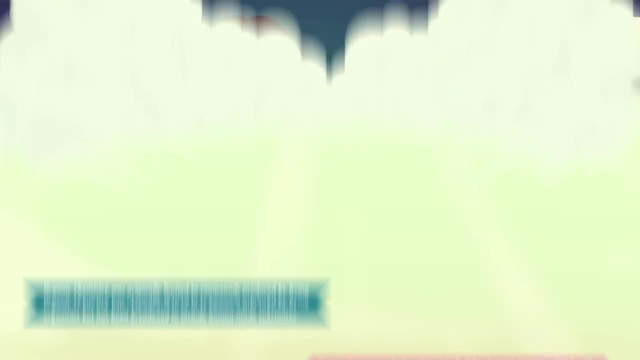 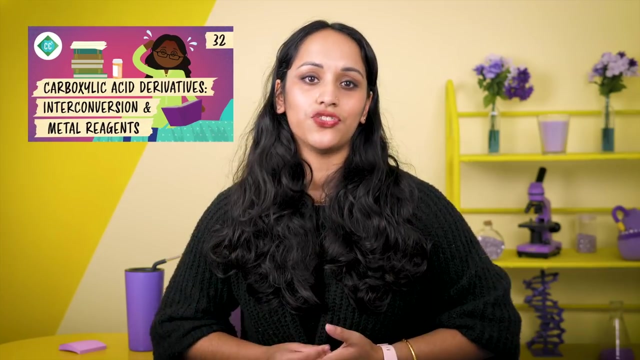 but it's technically called a protecting group. In this episode we'll learn how we can use protecting groups to control how our molecules react. In episode 32, we saw how we can reduce carbonyl compounds using metal hydrides. This is really straightforward if we have a molecule with just one carbonyl group.